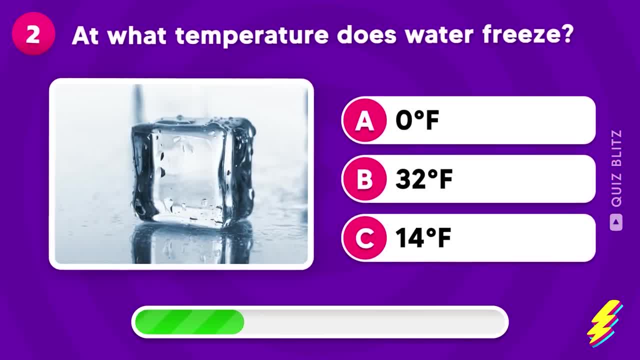 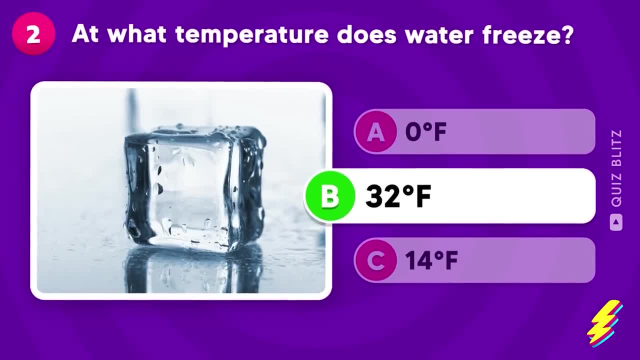 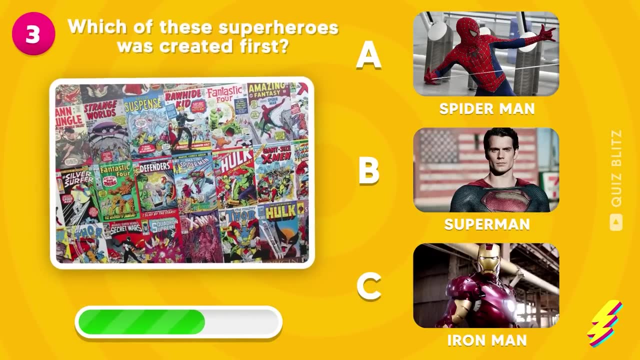 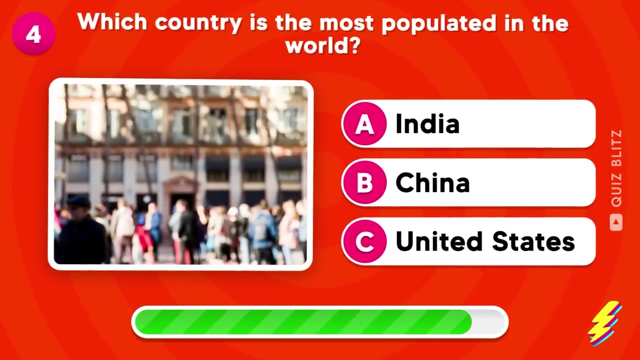 32°C or 0°C? Which of these superheroes was created first- Spider-Man, Superman or Iron Man? It's Superman. He was created in 1933.. Which country is the most populated in the world? India, China or United States? 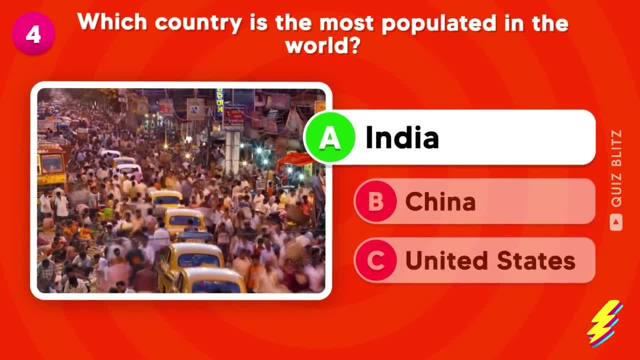 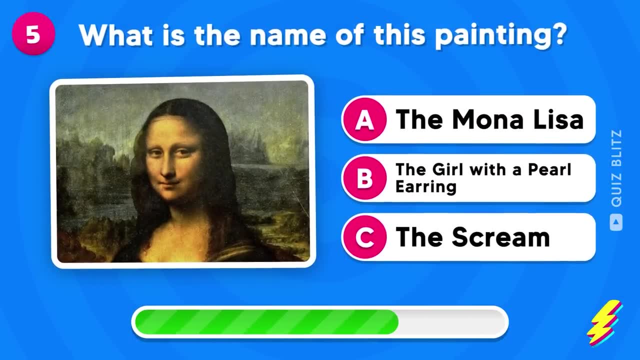 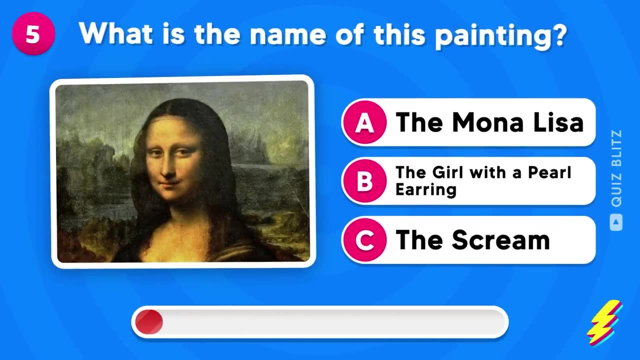 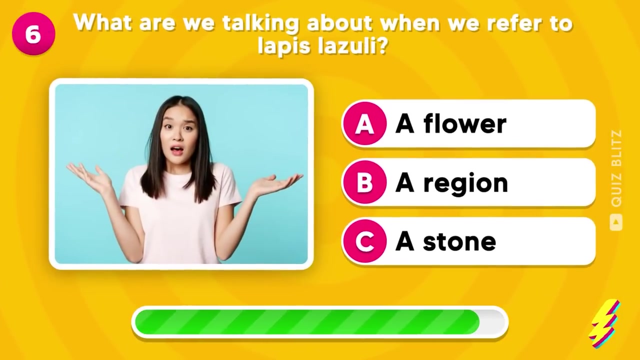 It's India, with over 1.4 billion inhabitants, closely followed by China. What is the name of this painting? The Mona Lisa, the girl with a pearl earring? or the scream: You've got this. The Mona Lisa. What are we talking about when we refer to lapis lazuli- A flower, a region or a stone? 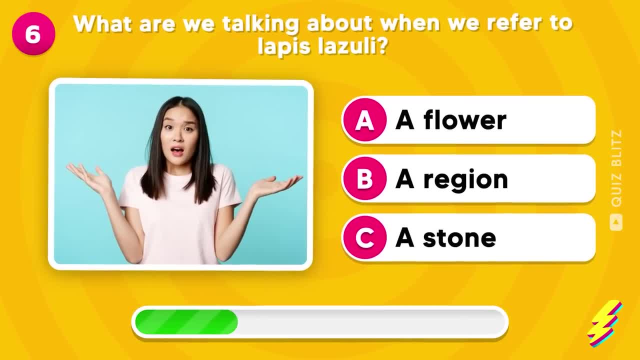 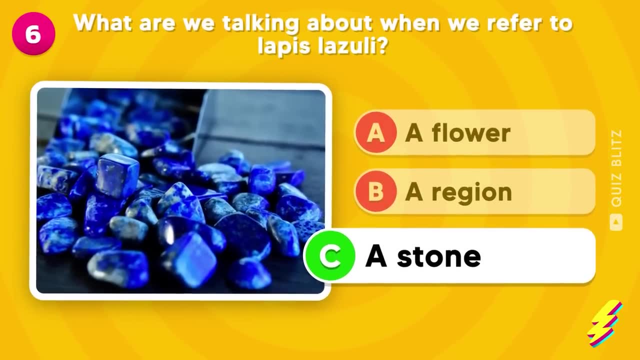 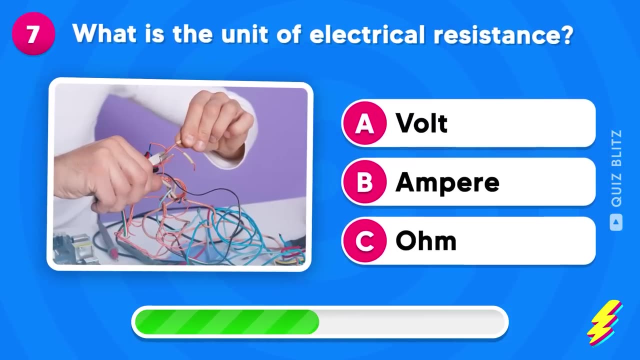 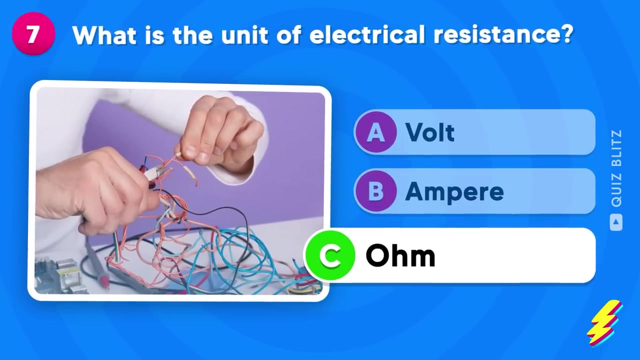 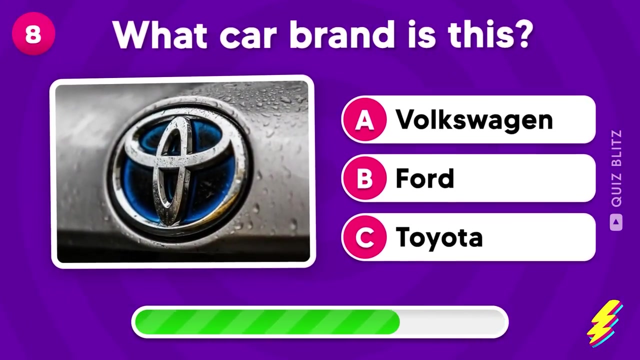 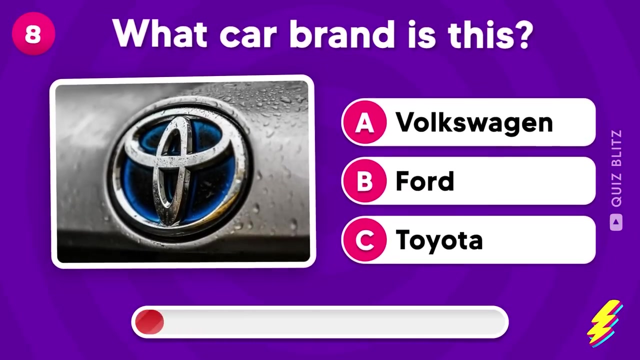 What's your pick? What are we talking about when we refer to lapis lazuli- A flower, a region or a stone? What's your pick? it's a stone. what is the unit of electrical resistance- volt, ampere or own? what car brand is this? Volkswagen, Ford or Toyota? Toyota, very good. how many faces does 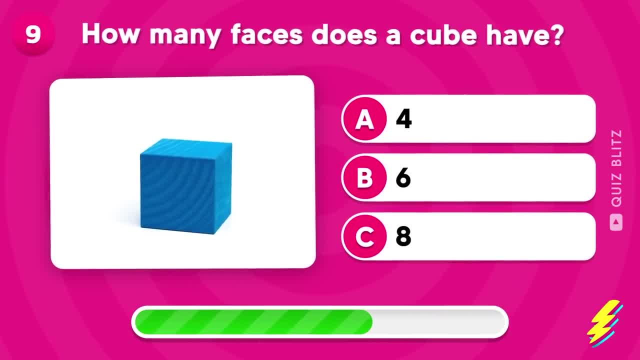 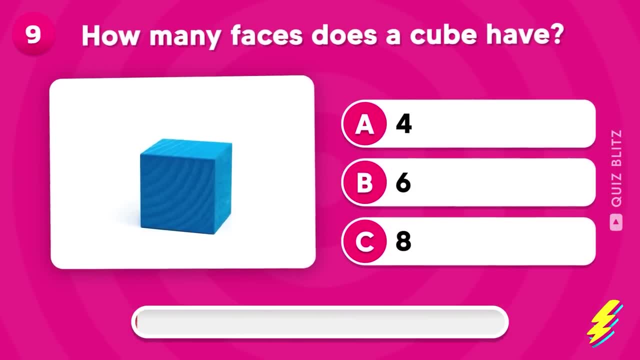 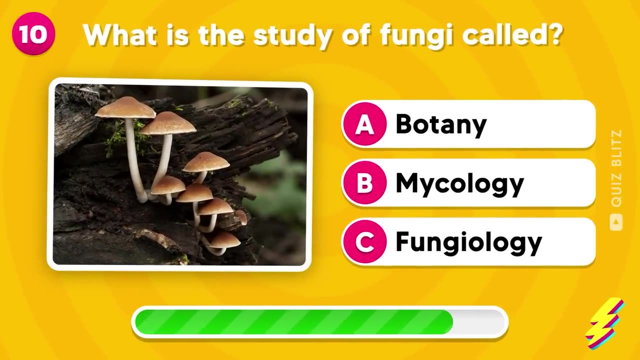 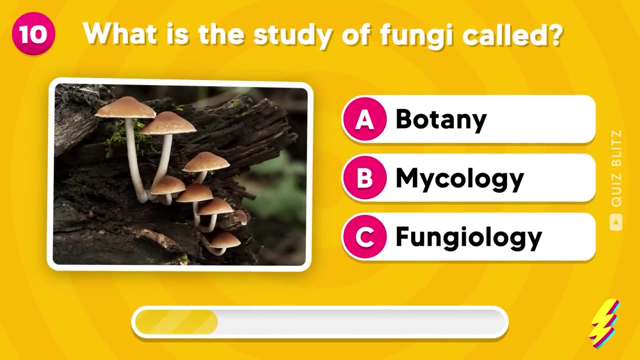 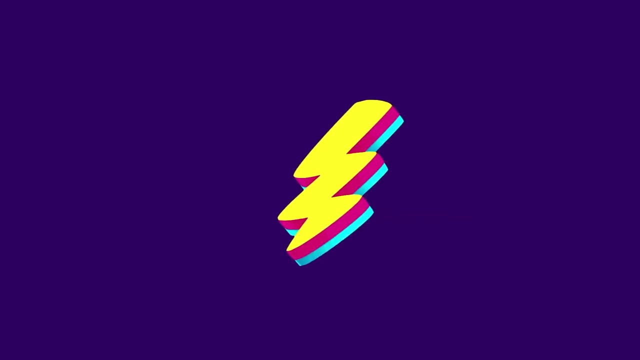 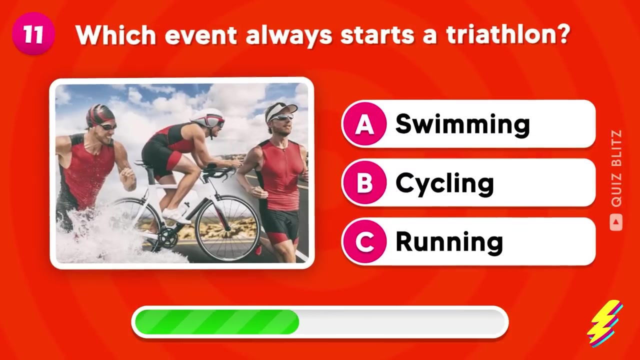 a cube have on it. what is the unit of electrical resistance? volt, ampere or own? have 4, 6 or 8, 6? what is the study of fungi called botany, mycology or fun geology? it's mycology which event always starts a triathlon, swimming, cycling or running? it's. 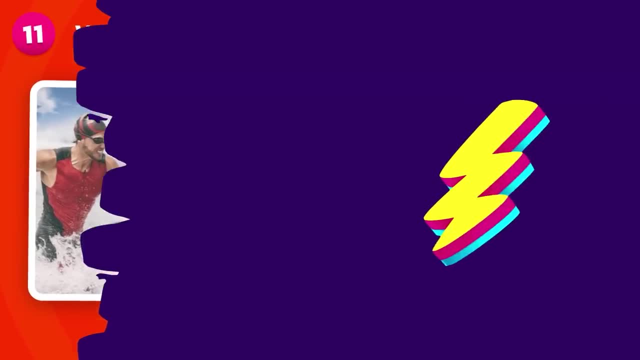 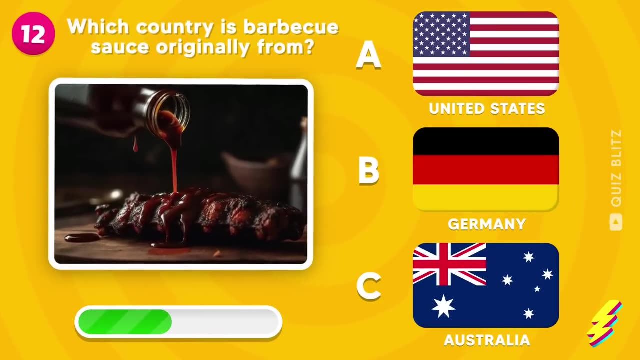 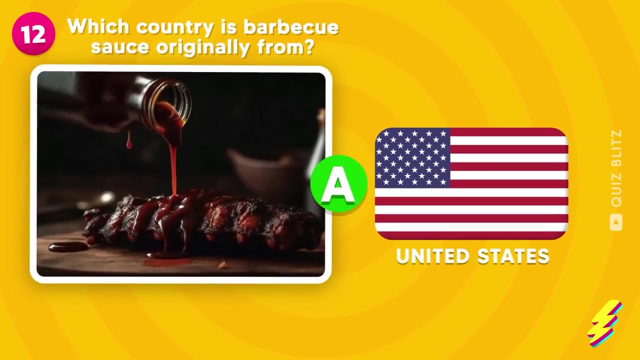 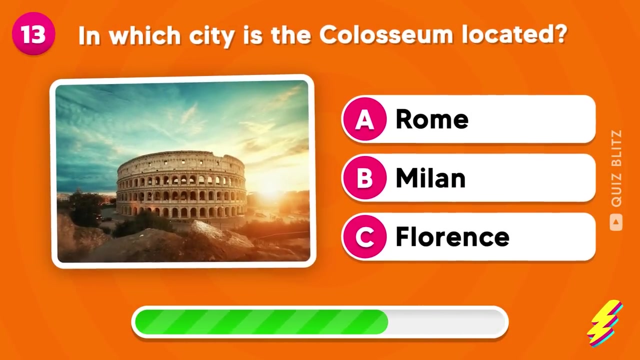 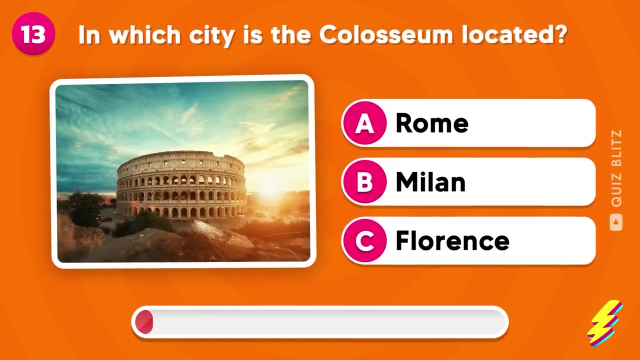 swimming, followed by cycling, then running. which country is barbecue sauce originally from United States, Germany or Australia? you, it comes from the United States. in which city is the Coliseum located? Rome, Milan or Florence? the Coliseum is located in Rome. how many days are there in a leap? 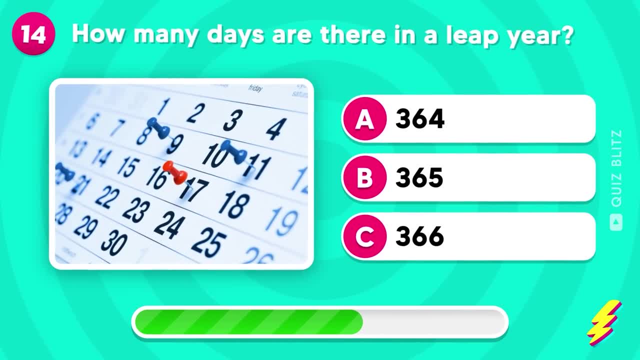 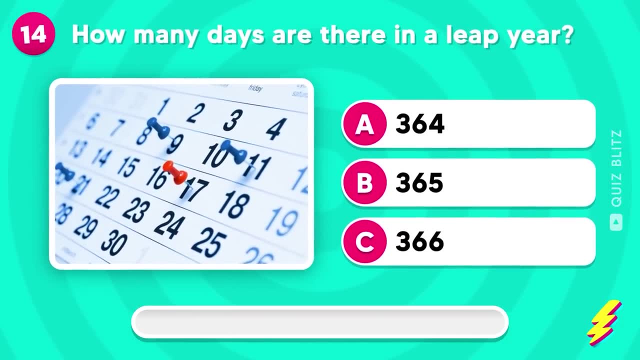 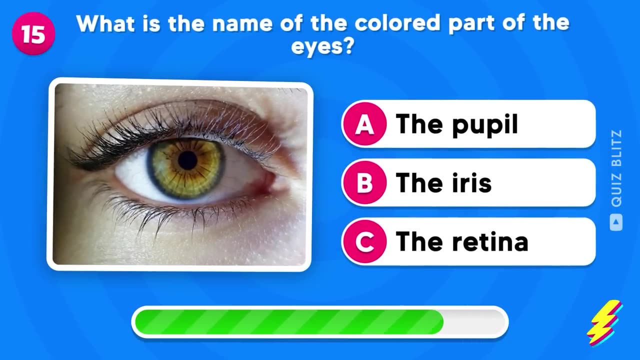 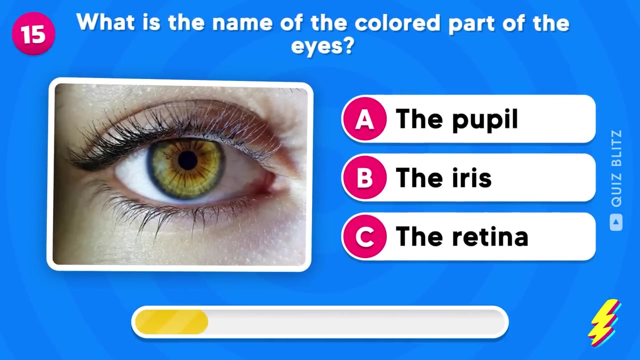 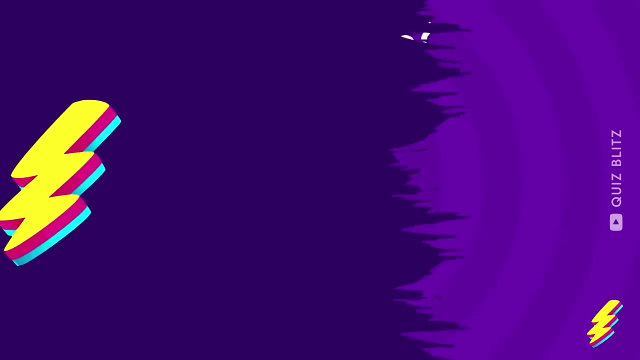 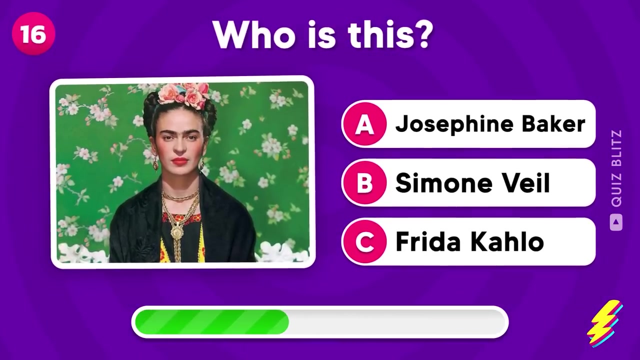 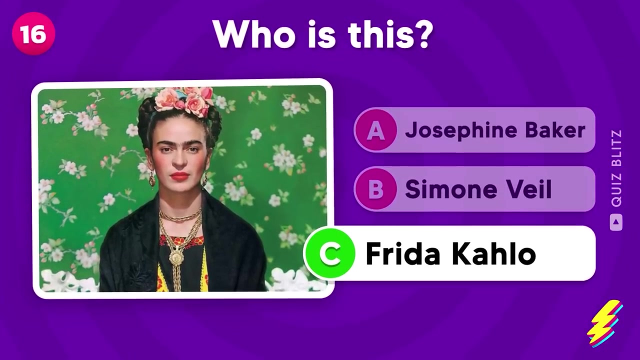 year 364, 365 or 366? what is the name of the colored part of the eyes, the pupil, the iris or the retina? it's the iris. who is this? Josephine Baker, Simone Weil? you are free to colo. Frida Kahlo, What is the official language of Egypt? 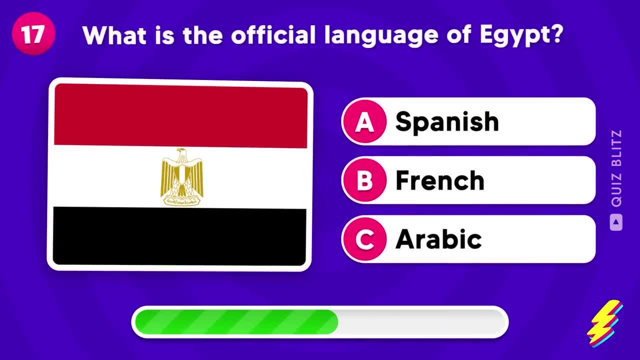 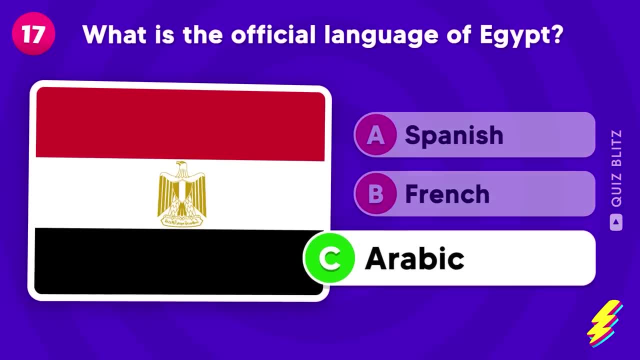 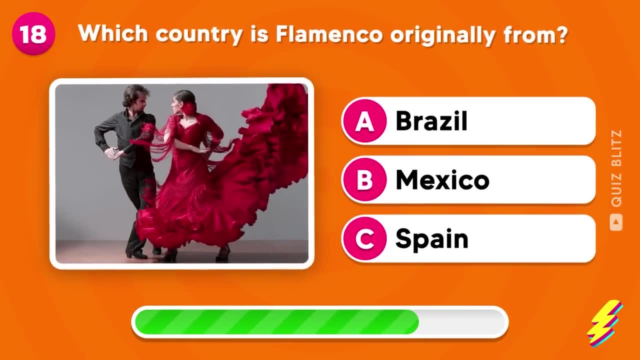 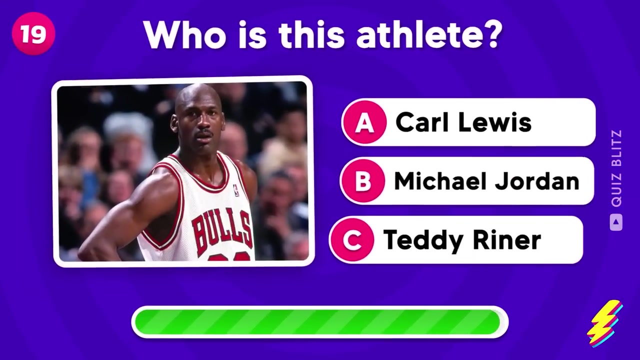 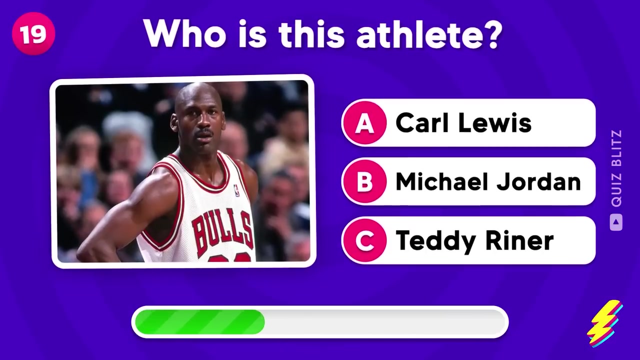 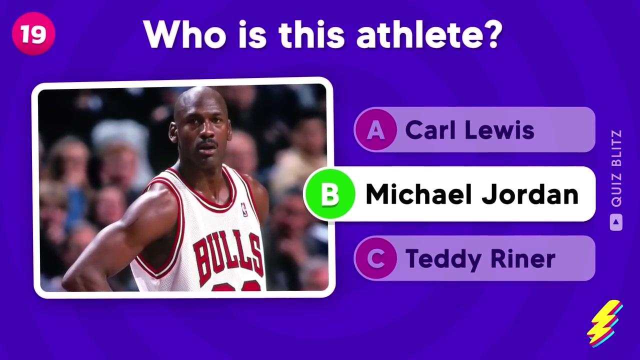 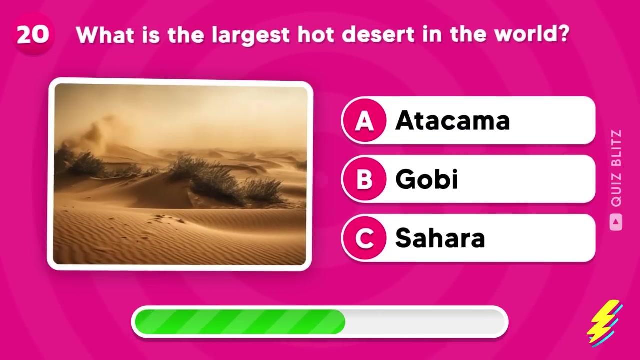 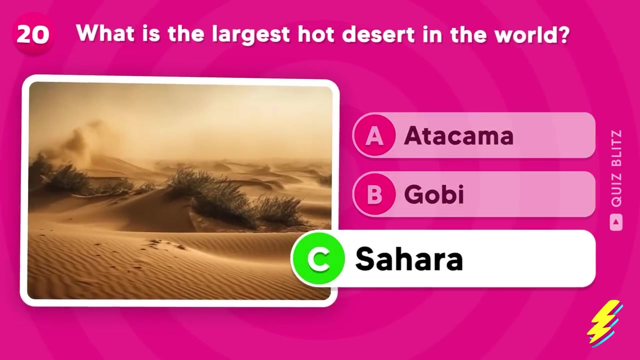 Spanish, French or Arabic? Arabic, Incredible. Which country is flamenco originally from? Brazil, Mexico or Spain, Spain? Who is this athlete? Carl Lewis, Michael Jordan or Teddy Ryan? Any ideas? Michael Jordan, What is the largest hot desert in the world? Atacama, Gobi or Sahara? 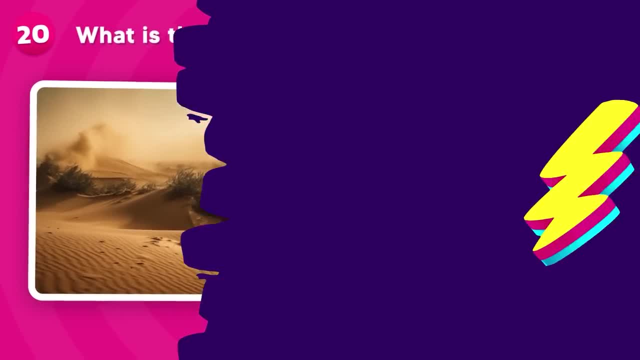 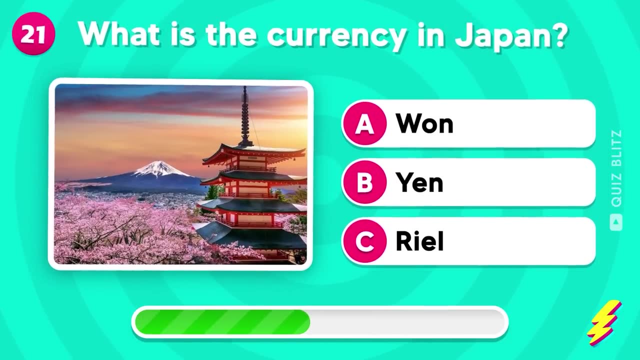 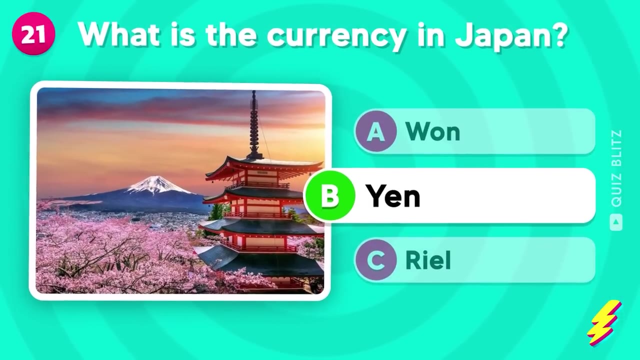 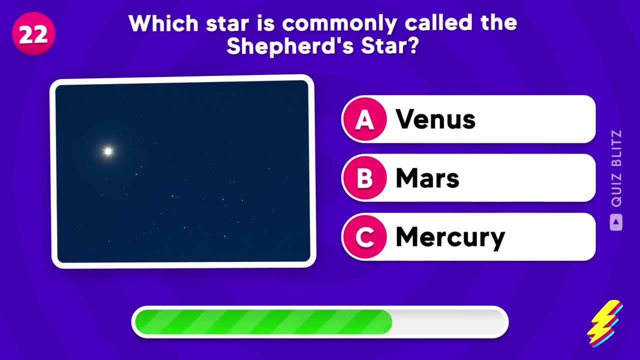 It's the Sahara Desert. What is the currency in Japan? Won Yen or Riel Japan. Japan, Japan The Yen. The Yen, The Yen. Which star is commonly called the Shepard's Star, Venus, Mars or Mercury? 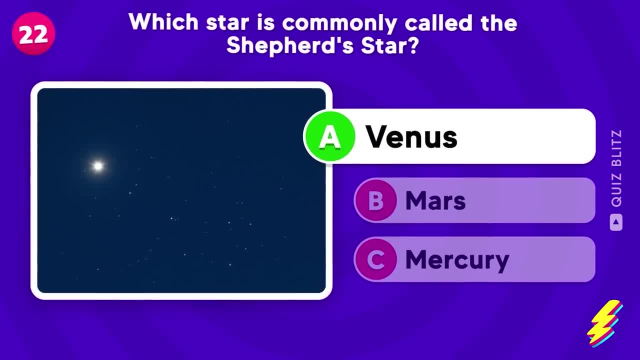 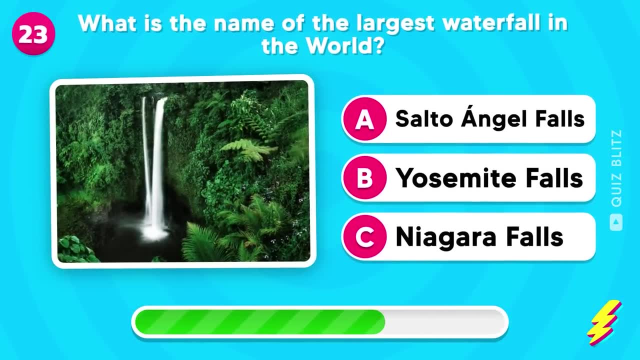 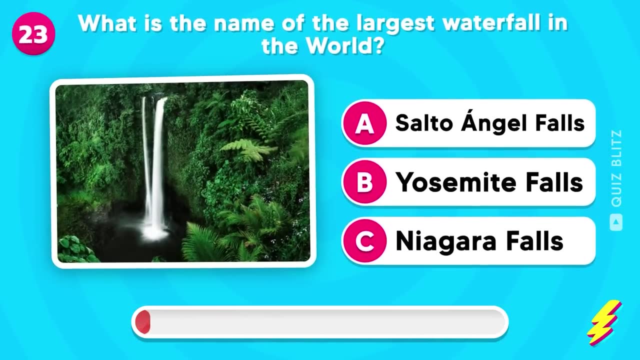 Venus. What is the name of the largest waterfall in the world? Answer A, B or C. Answer A, B or C. Answer A, B or C. Answer B: our headika Answer開始. The Salto Angel falls in Venezuela. 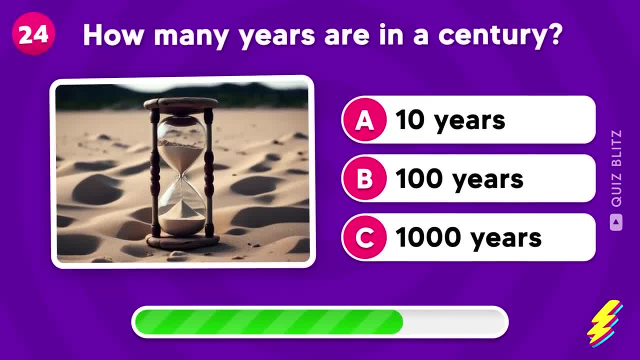 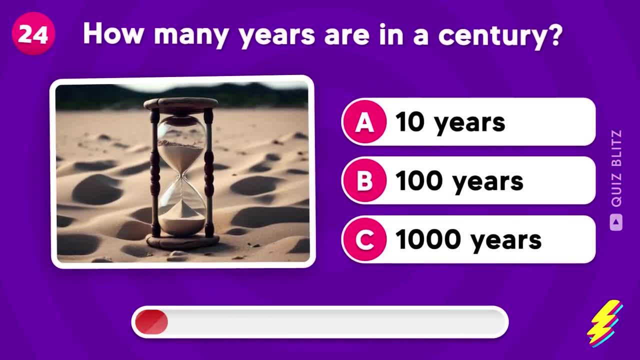 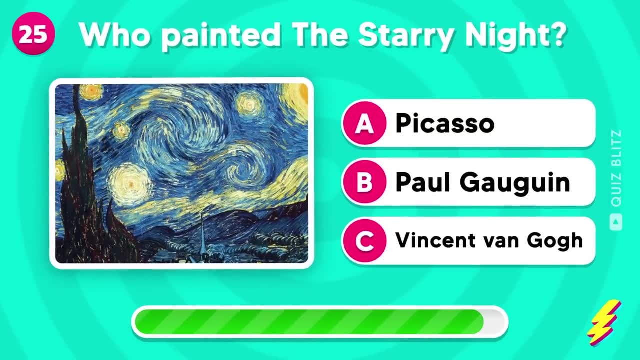 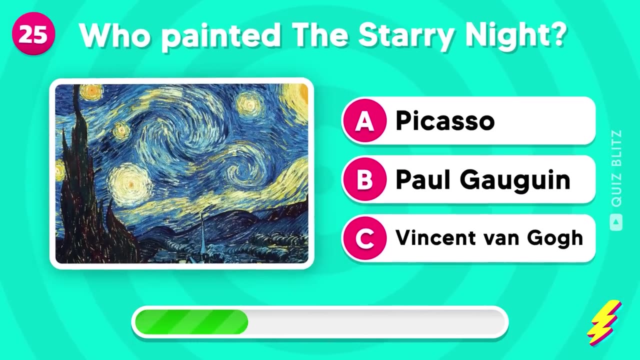 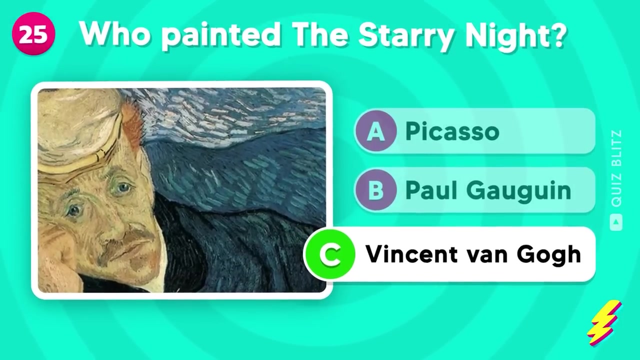 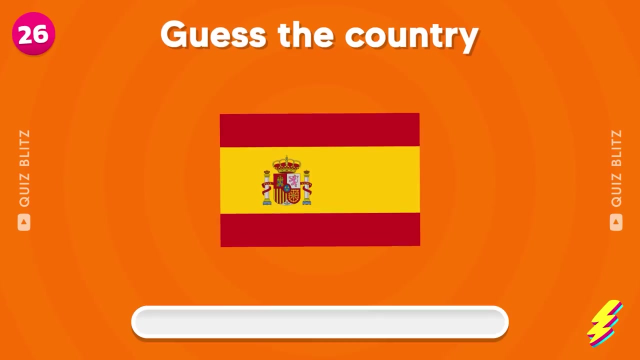 How many years are in a century? 10 years, 100 years or 1,000 years? Answer: Well spotted: it's 100 years. paul gauguin or vincent van gogh? vincent van gogh? guess the country? it's spain. 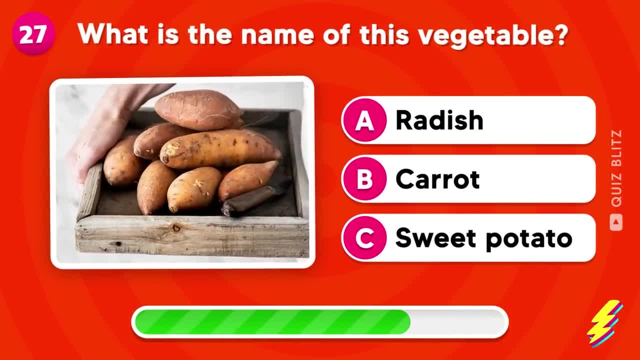 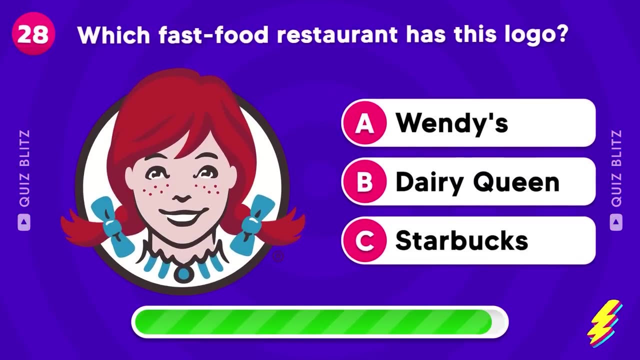 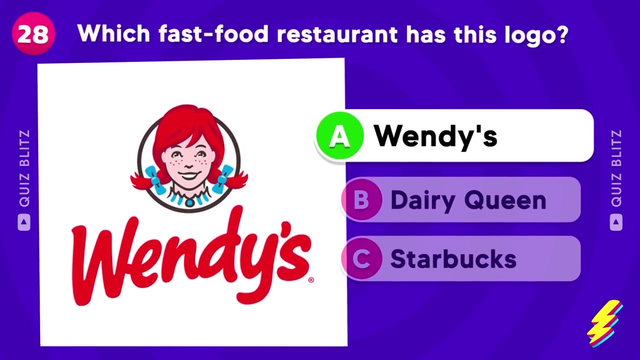 what is the name of this vegetable radish, carrot or sweet potato? yes, those are sweet potatoes. which fast food restaurant has this logo? wendy's dairy queen? or starbucks wendy's very good? who painted the famous mural on the ceiling of the sistine? 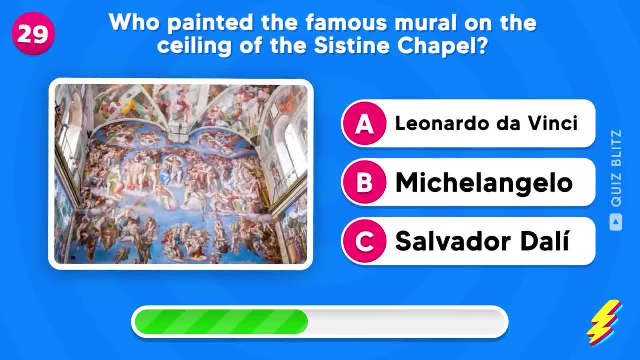 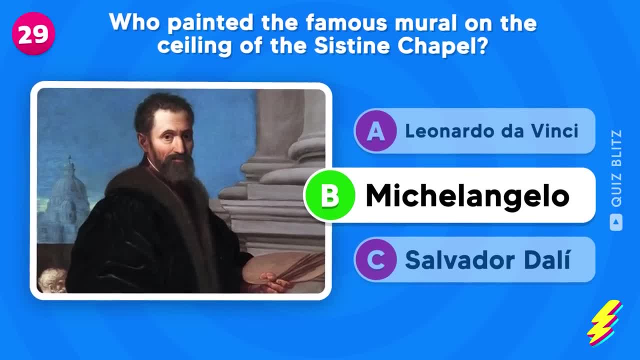 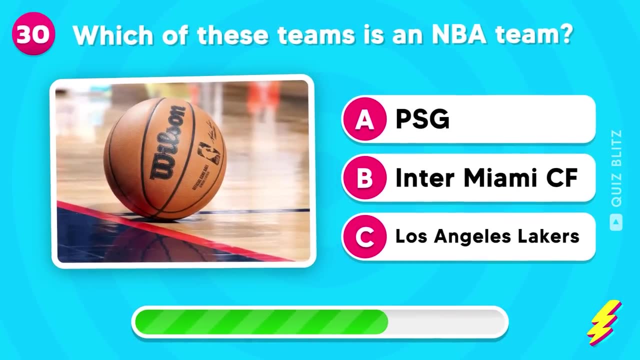 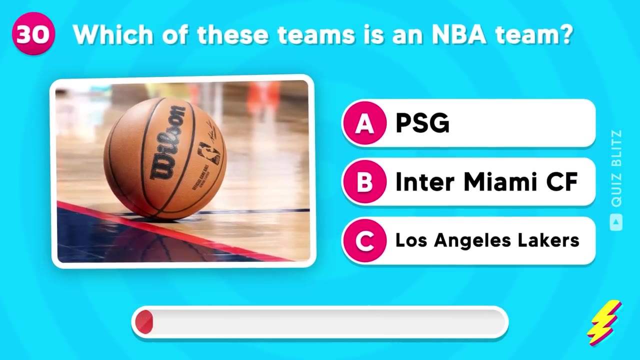 chapel, leonardo da vinci, michelangelo or salvador dali, michelangelo? which of these teams is an nba team? psg enter miami cf or los angeles lakers. los angeles lakers. very good, let's go Continue. 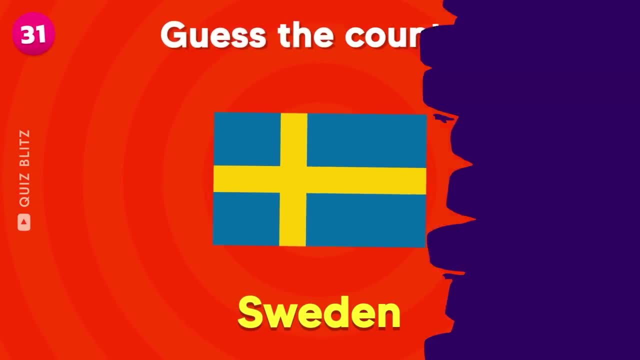 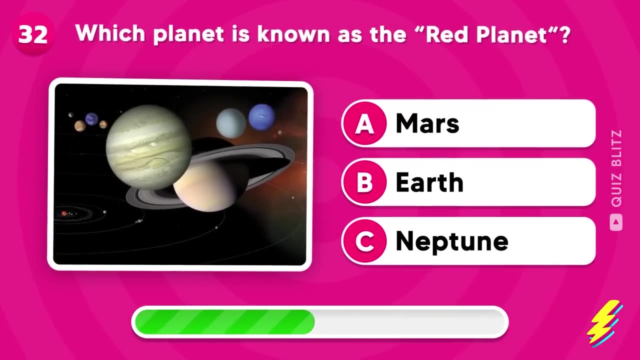 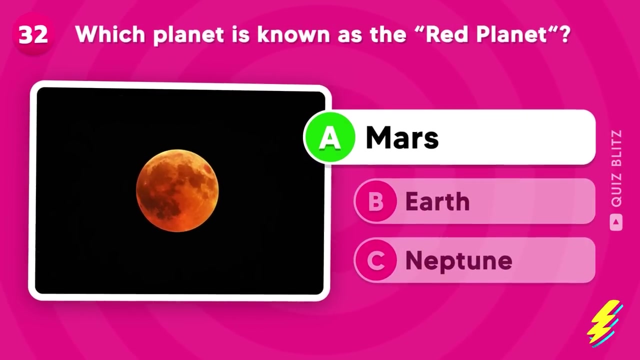 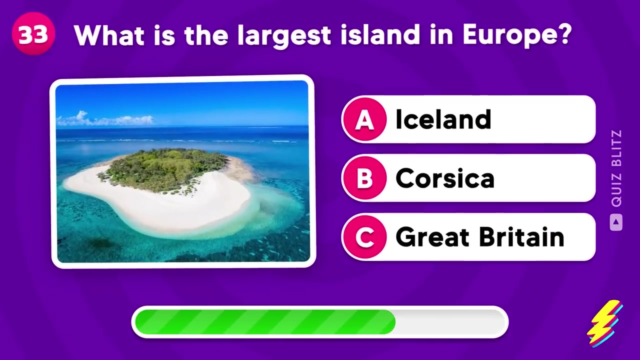 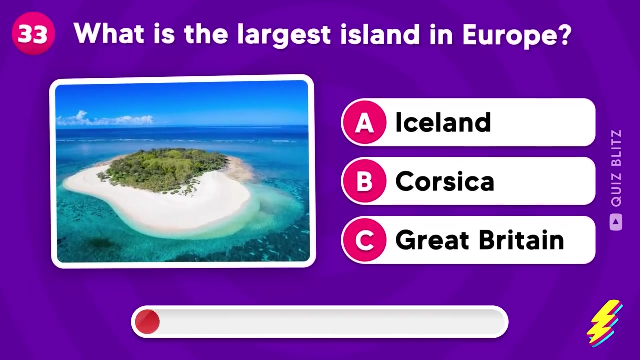 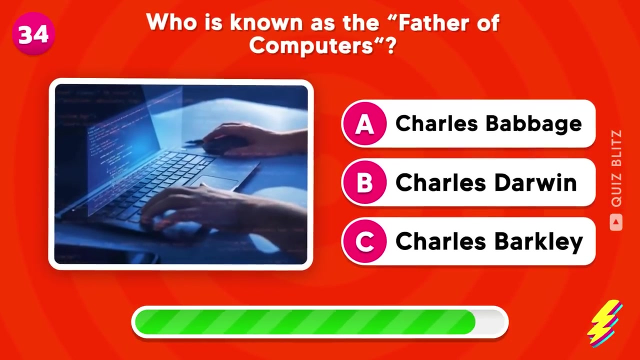 Sweden. Which planet is known as the Red Planet, Mars, Earth or Neptune? It's Mars. What is the largest island in Europe- Iceland, Corsica or Great Britain? Great Britain, Who is known as the father of computers? 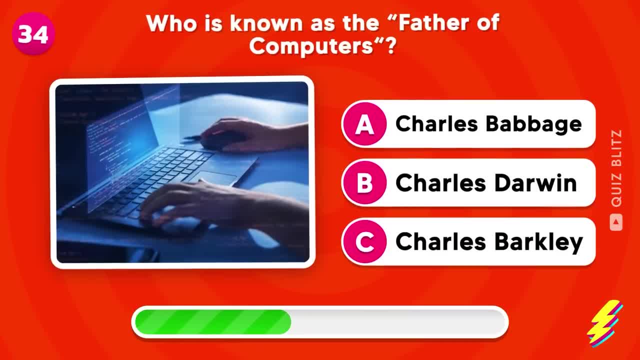 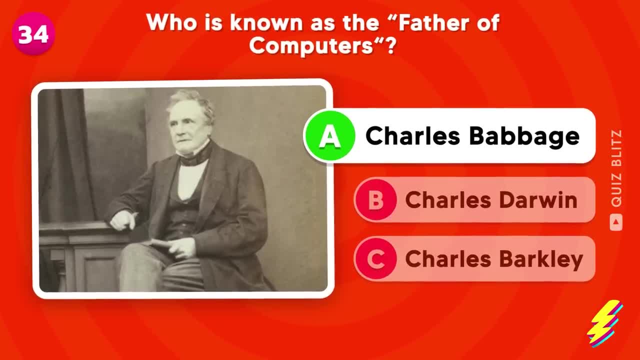 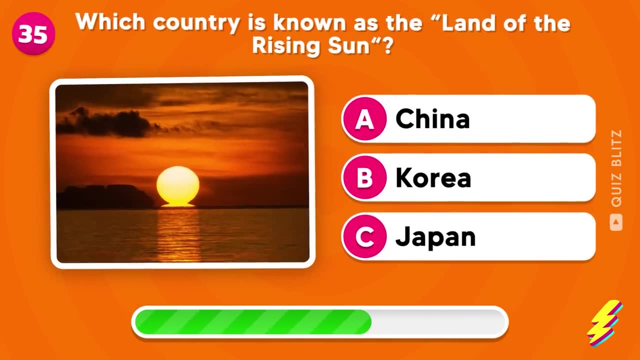 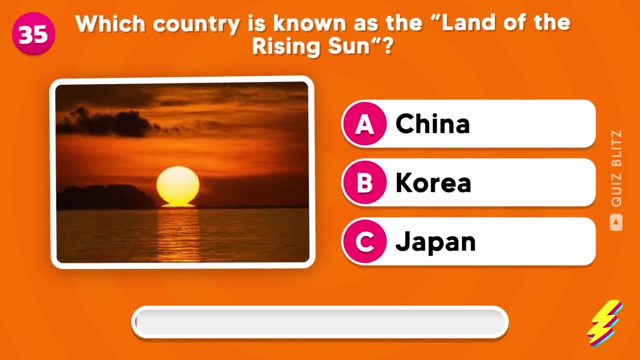 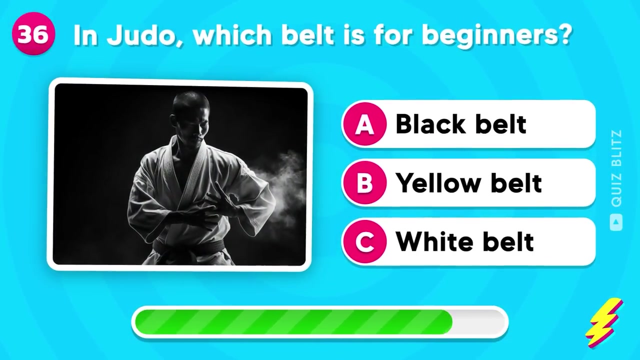 Charles Babbage? Charles Darwin or Charles Barkley? And yes, it's Charles Babbage. Which country is known as the Land of the Rising Sun? China, Korea or Japan? Japan In judo. which belt is for beginners? 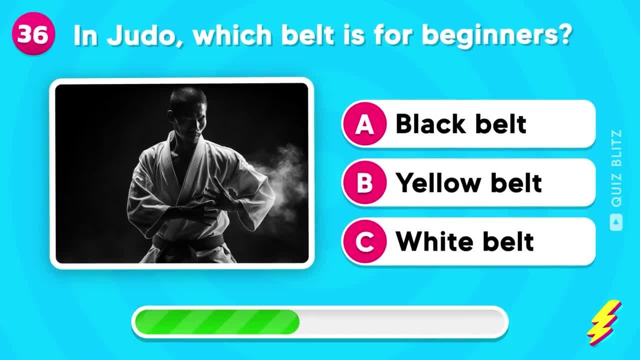 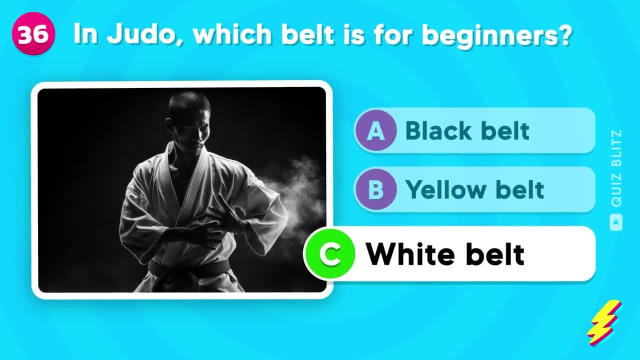 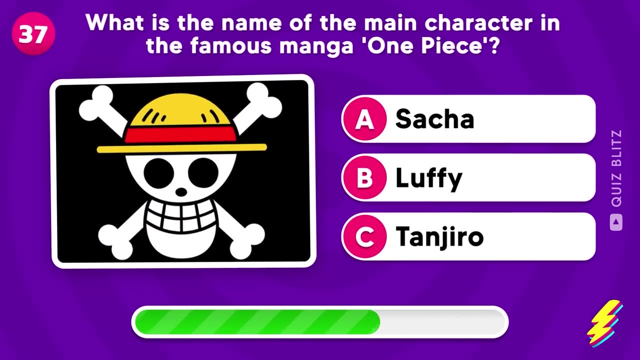 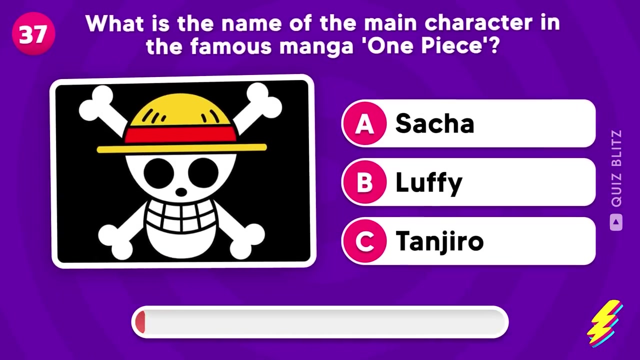 Black belt, yellow belt or white belt? It's the white belt. What is the name of the main character in the famous manga One Piece? Sasha, Luffy or Tanjiro? It's Luffy Who wrote Romeo and Juliet. 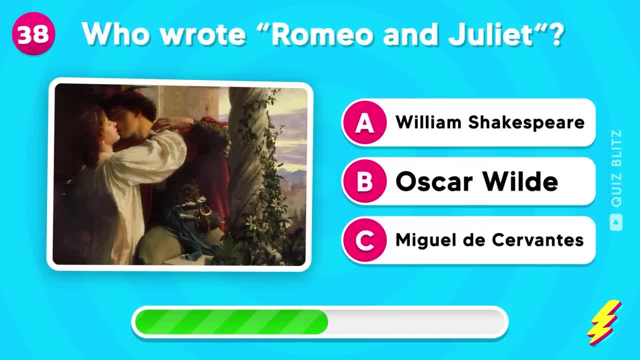 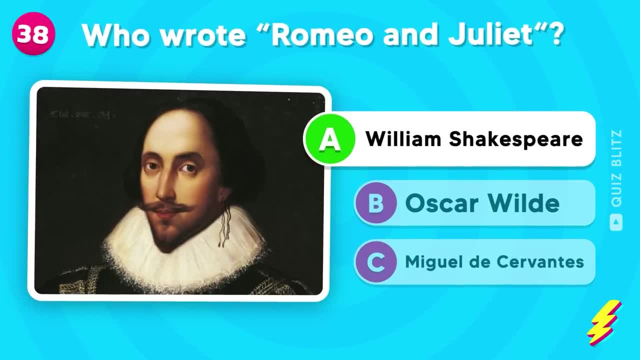 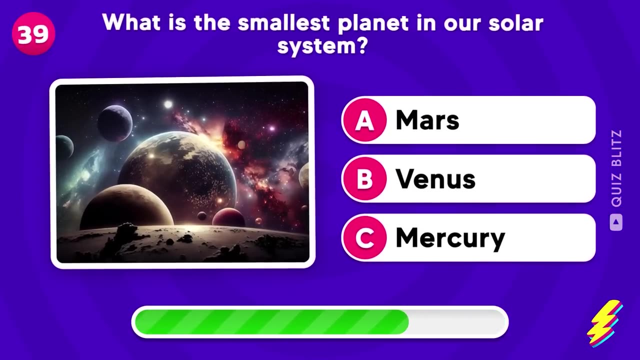 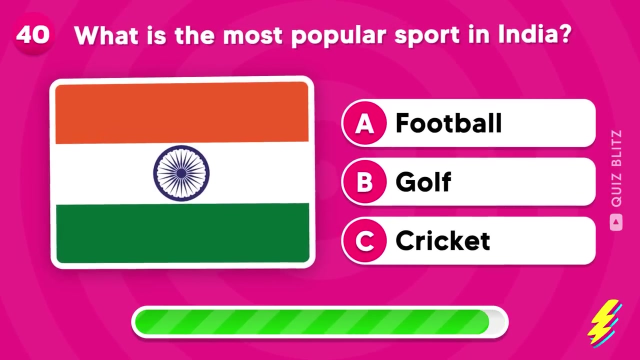 William Shakespeare, Oscar Wilde or Miguel de Cervantes? William Shakespeare, What is the smallest planet in our solar system? Mars, Venus or Mercury? Mars, Venus or Mercury? Well done, it's Mercury. What is the most popular sport in India? 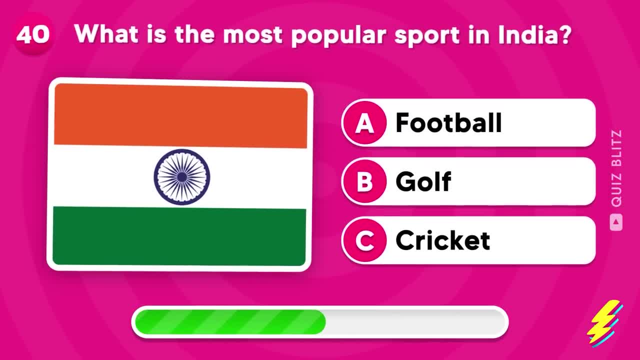 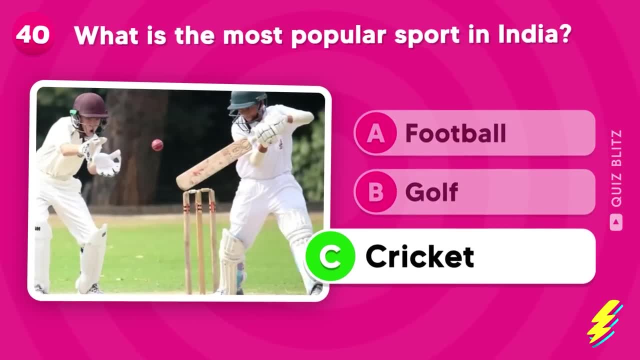 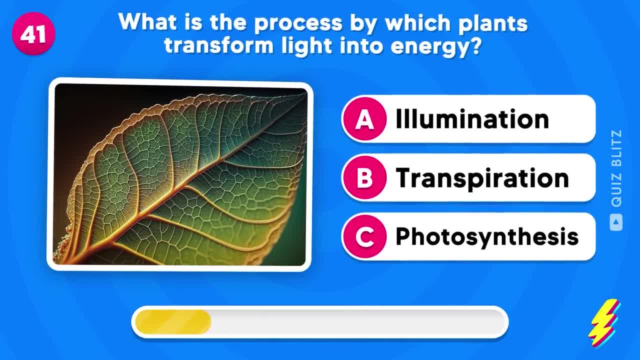 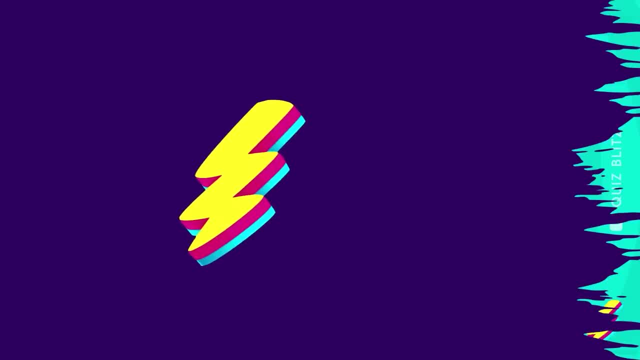 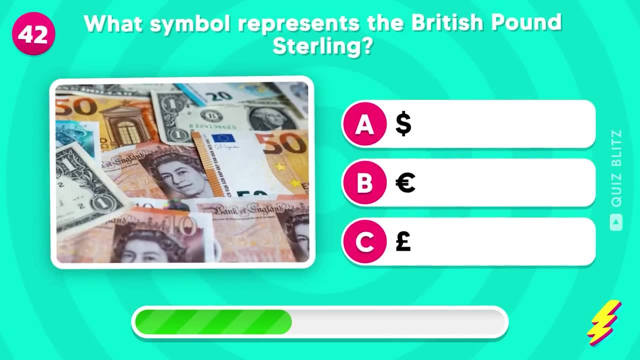 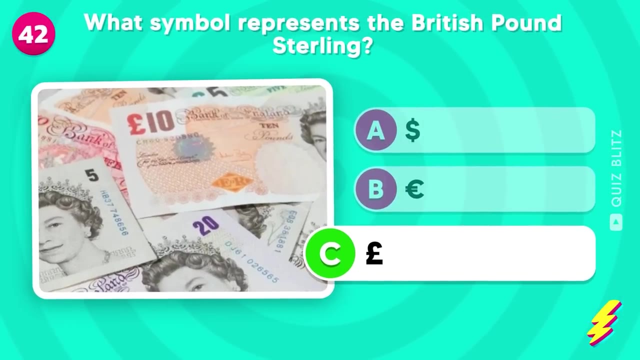 What is the process by which plants transform light into energy: Illumination, transpiration or photosynthesis. Photosynthesis: What symbol represents the British Pound sterling? What symbol represents the British Pound sterling, You're right. Which year marks the creation of printing and the printing of the first book? 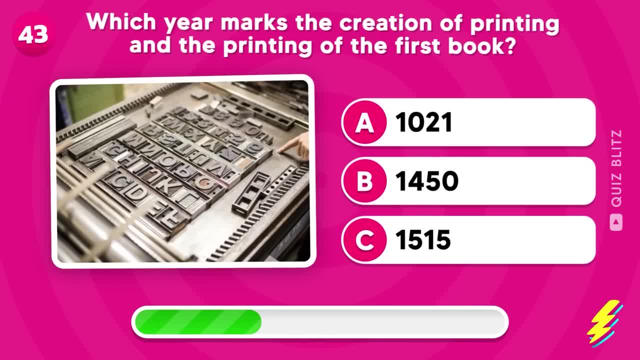 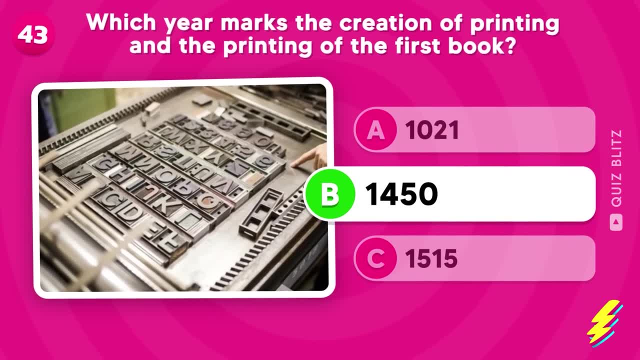 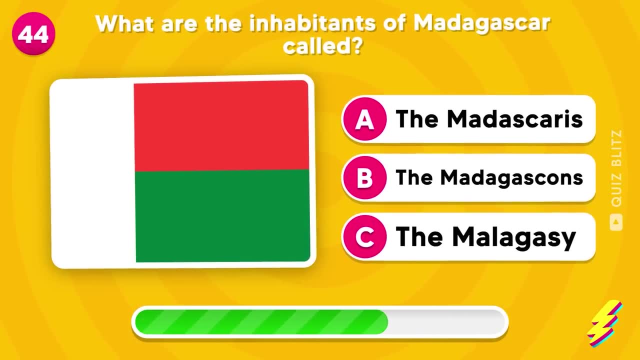 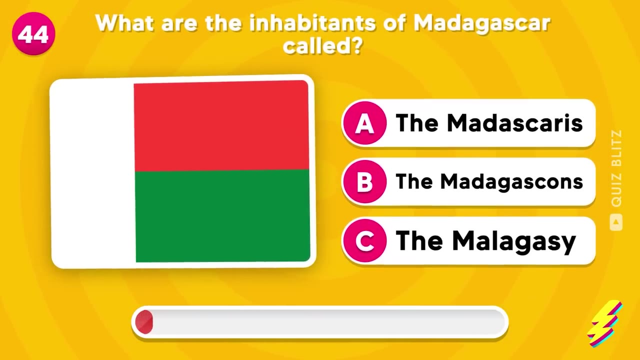 Answer A, B or C. The invention of printing dates back to 1450.. I wasn't even born then. What are the inhabitants of Madagascar, called The Matascares, the Madagascans, or the Malagasy, The Malagasy? incredible. 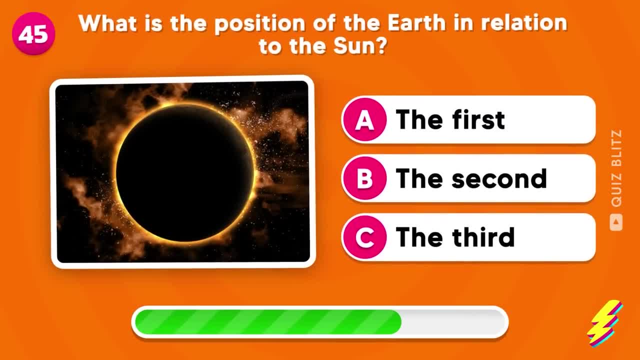 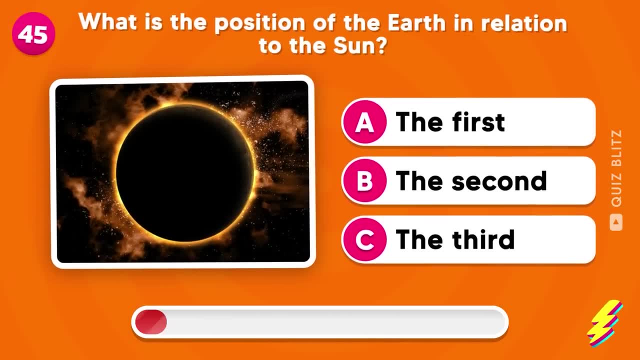 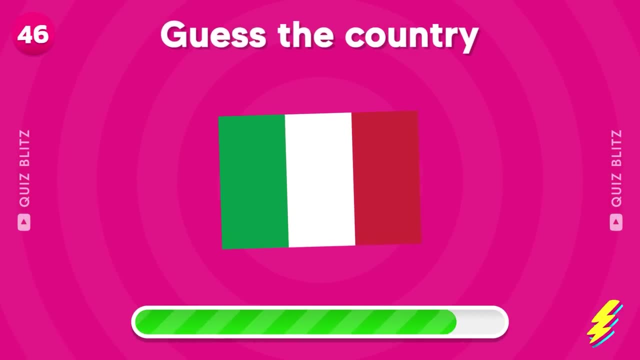 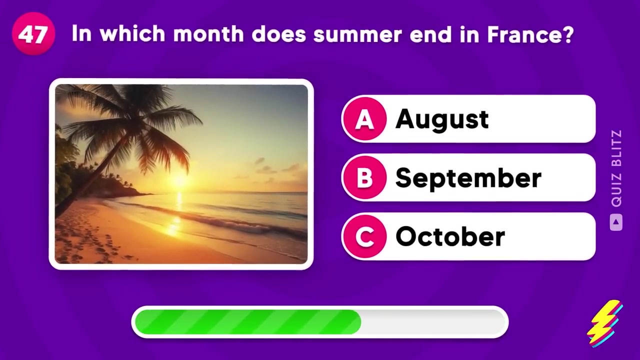 What is the position of the Earth in relation to the Sun? The first, the second or the third Answer: B, C or C? It's the third planet, after Mercury and Venus. Guess the country? It's Italy. In which month does summer end in France? August, September or October? 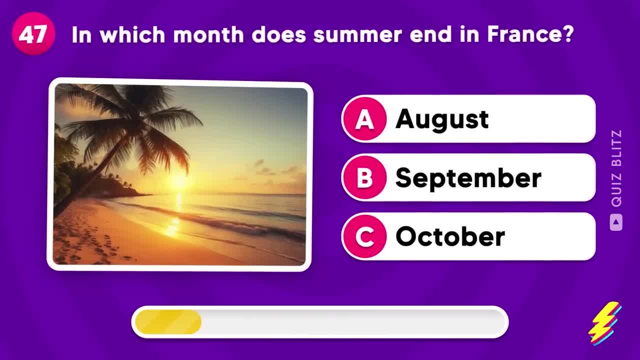 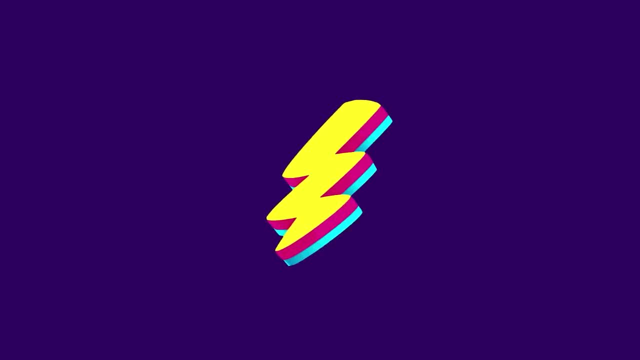 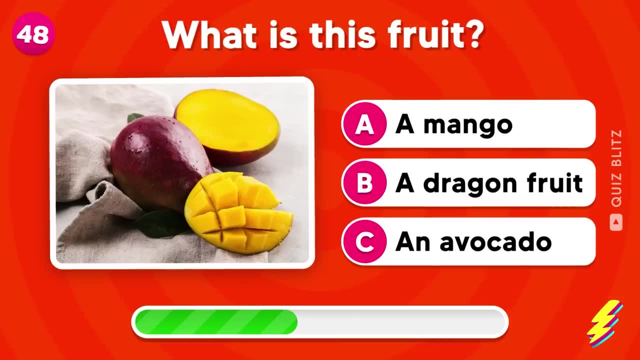 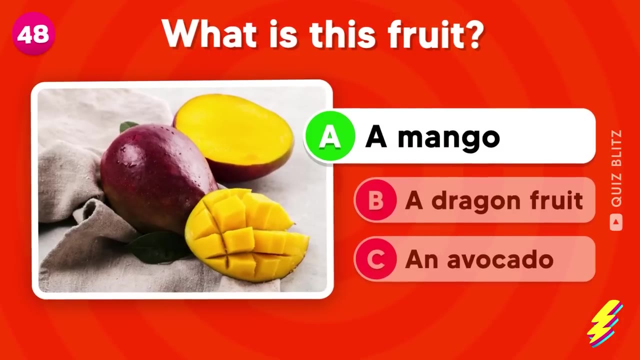 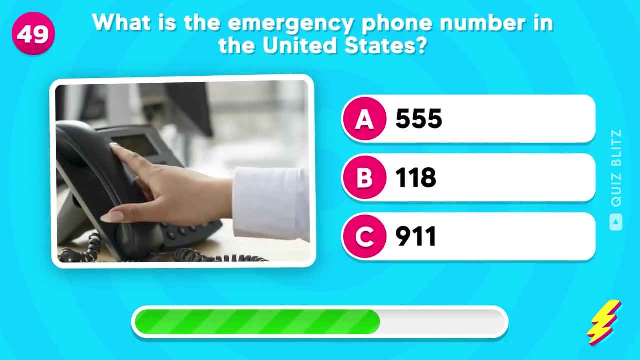 Answer C, C or C. Yes. Yes, It ends on September 21.. What is this fruit? A mango, a dragon fruit or an avocado? A mango. What is the emergency phone number in the United States? Answer: A, B or C. 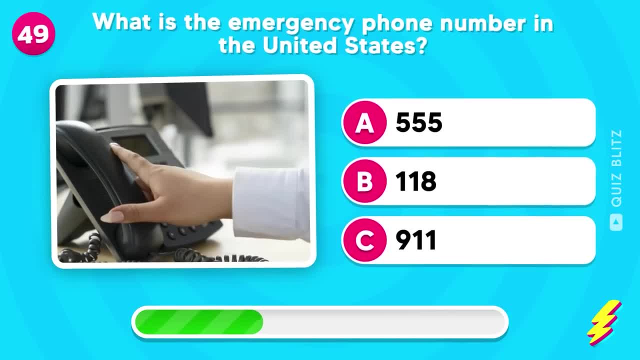 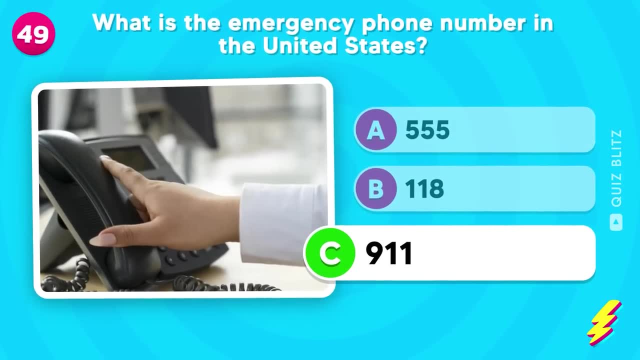 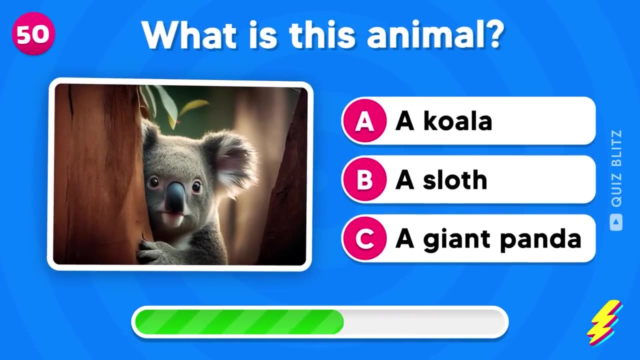 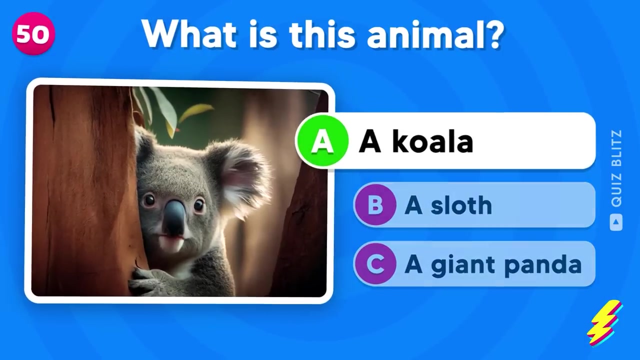 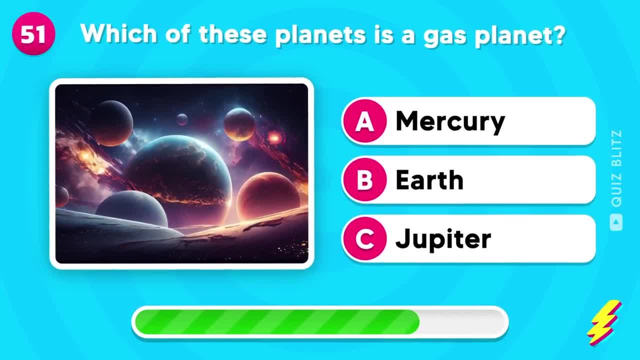 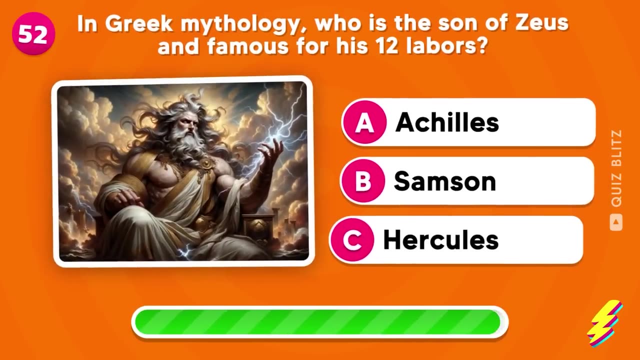 Which of these planets is a gas planet A, Mercury, Earth or Jupiter? Answer: D, C or E? Mars, Yes, Yes, B, C or V? Same answer. jupiter, incredible in greek mythology, who is the son of zeus and famous for his 12 labors. 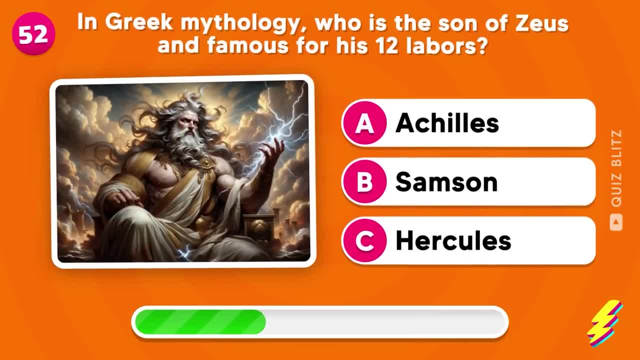 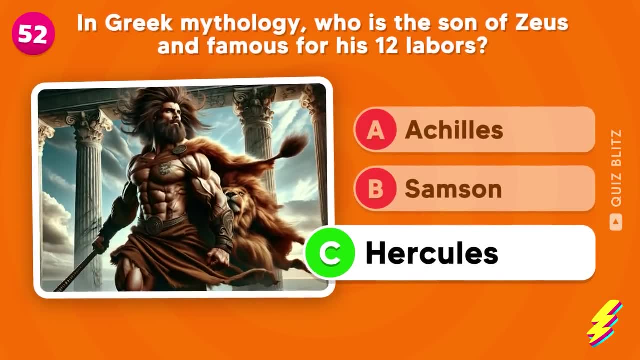 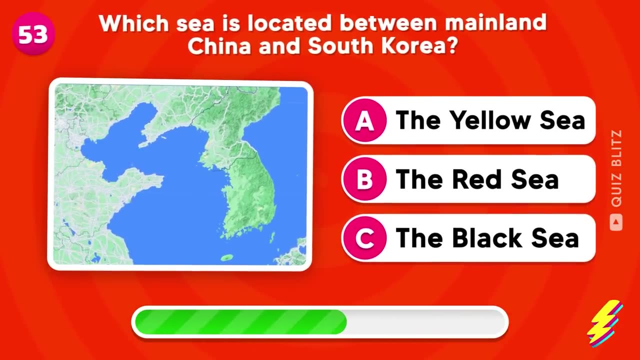 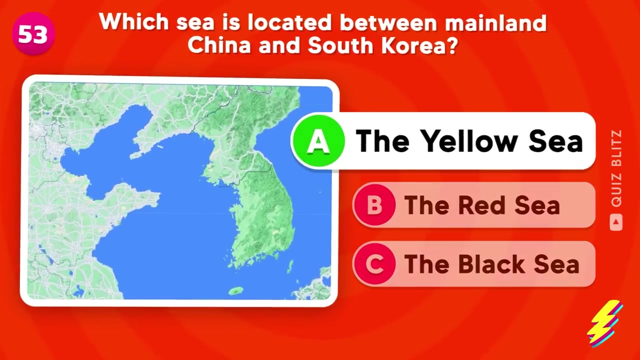 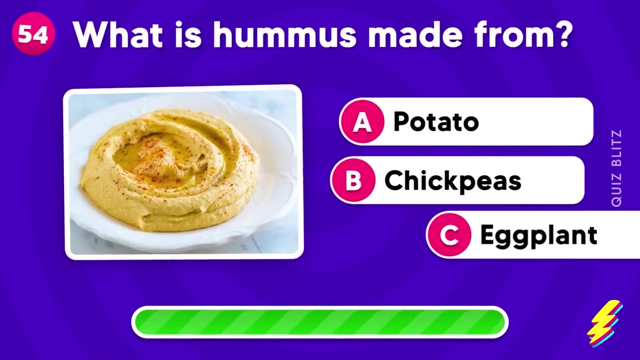 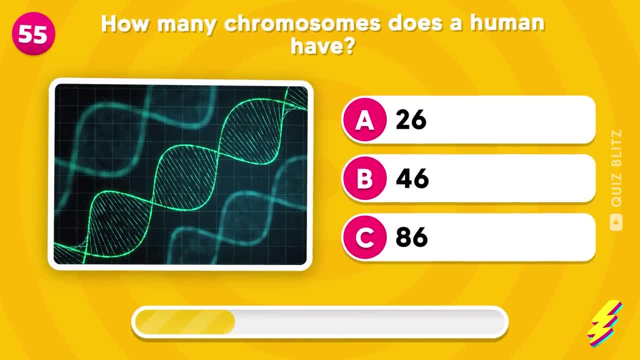 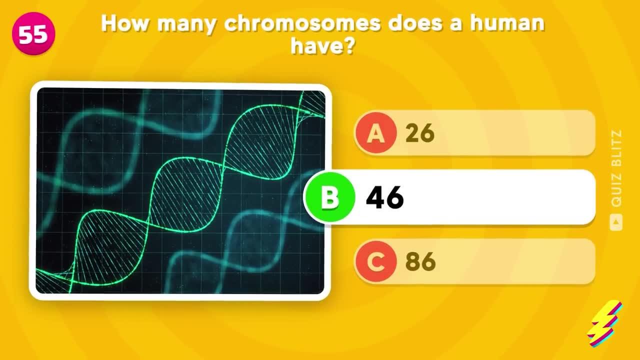 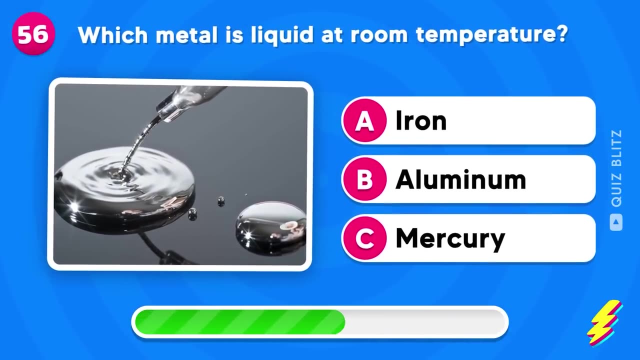 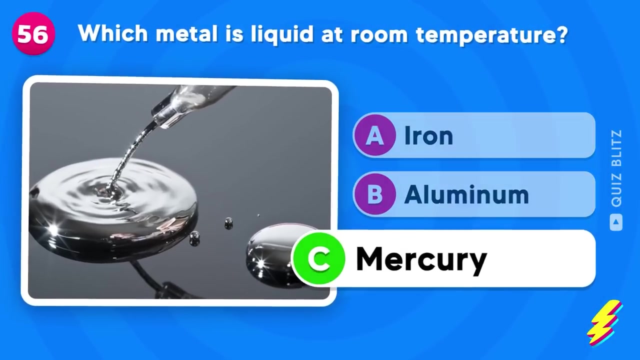 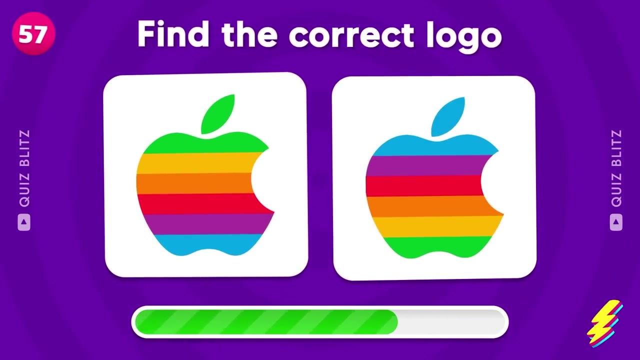 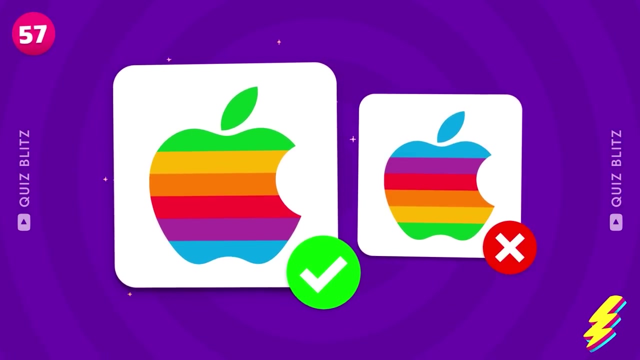 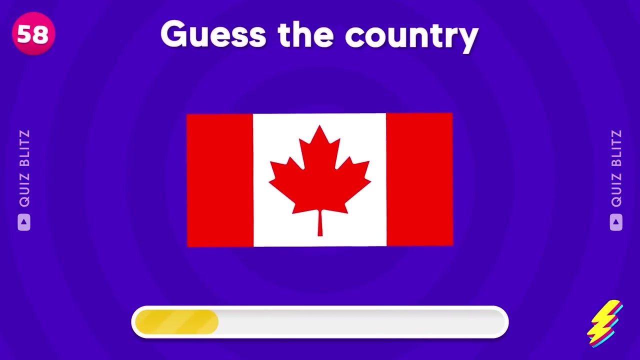 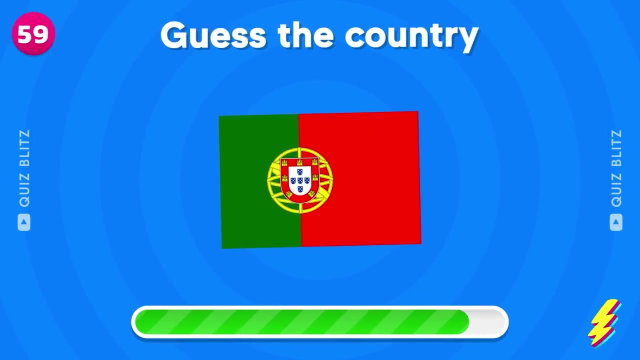 46. indeed, that makes 23 pairs. which metal is liquid at room temperature? iron, aluminum or mercury? 가요, What is the real Apple logo? This logo dates back to 1977.. It's the first one, Guess. the country, Canada, And this one? 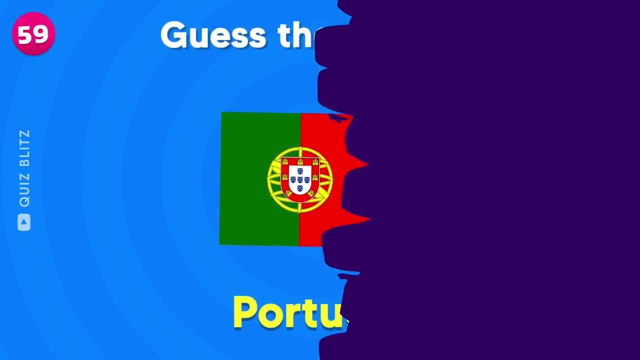 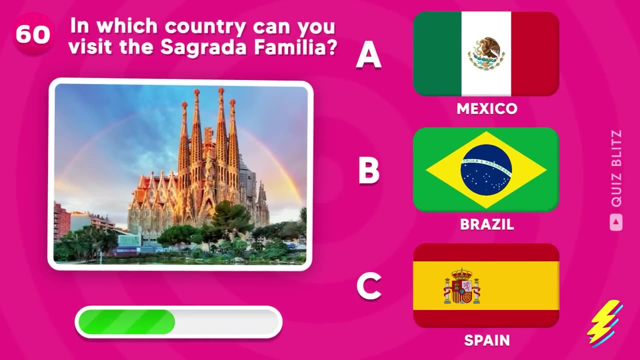 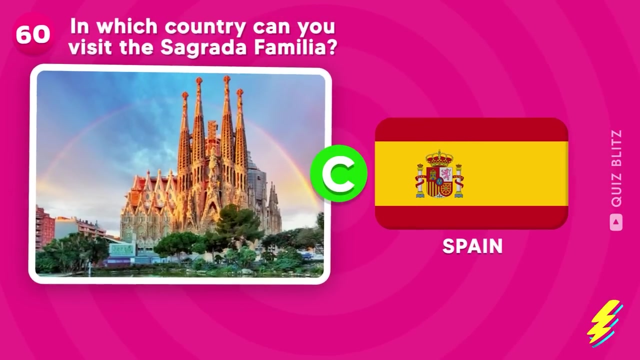 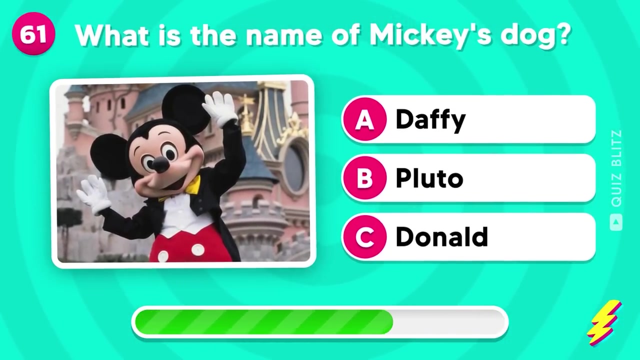 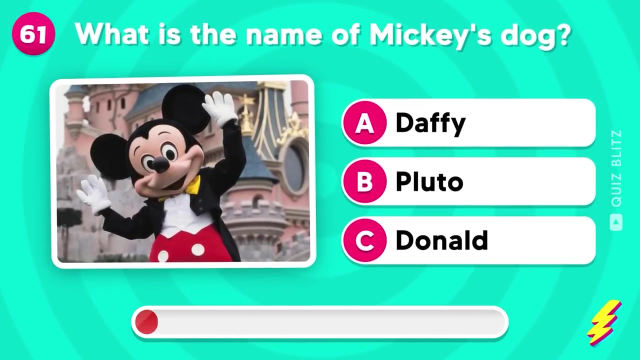 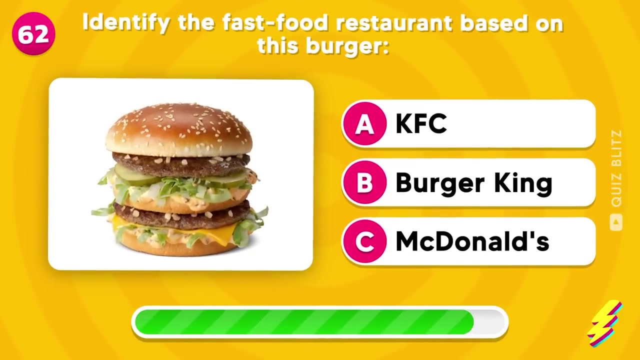 Portugal. In which country can you visit the Sagrada Familia? Mexico, Brazil or Spain, Spain? What is the name of Mickey's dog? Daffy, Pluto or Donald, Well done, It's Pluto. Identify the fast-food restaurant based on this burger: KFC, Burger King or McDonald's. 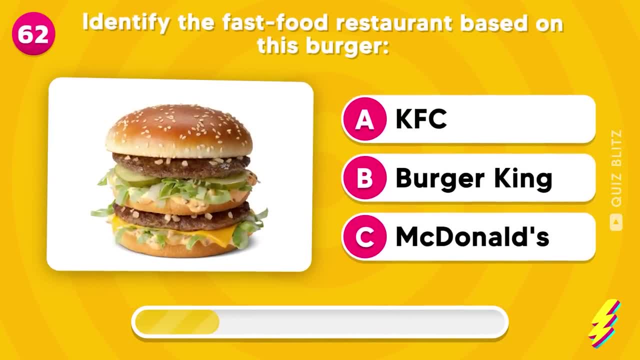 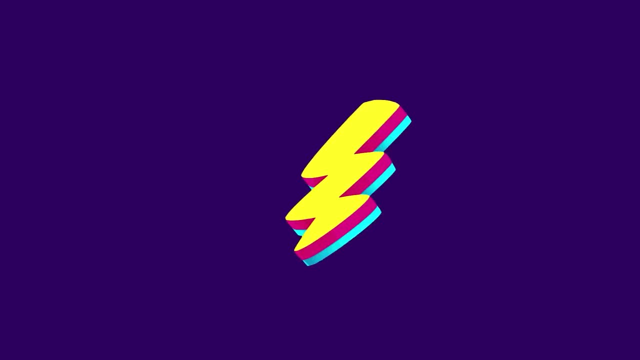 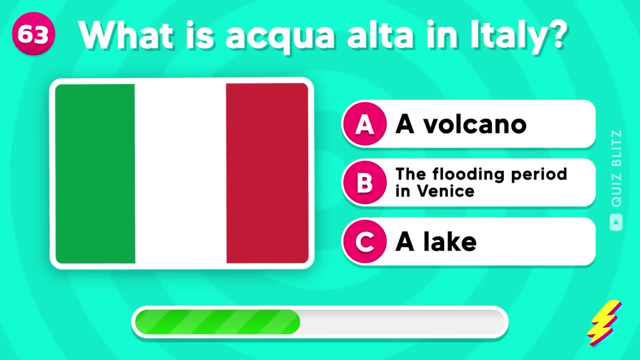 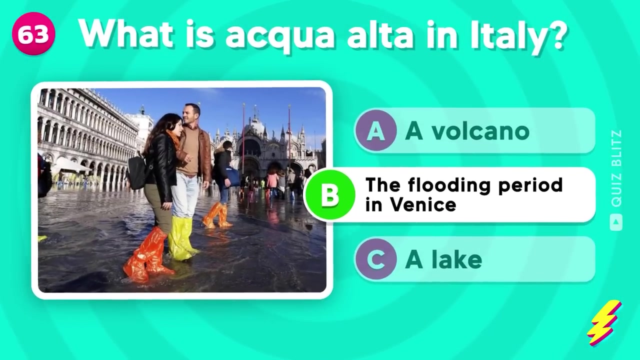 Spain? Yes, it's a Big Mac from McDonald's. What is Acqua Alta in Italy? A volcano, The flooding period in Venice, or a lake, The flooding period in Venice? Which chess piece can only move diagonally? The bishop. 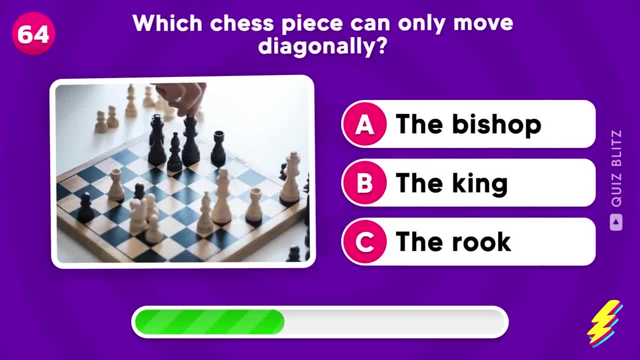 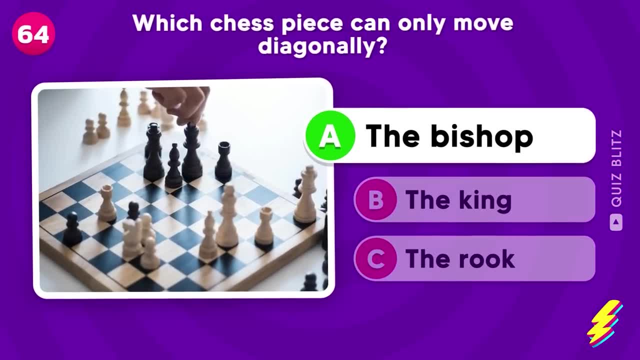 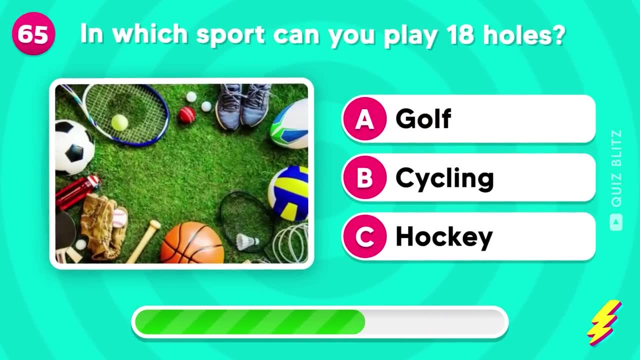 The king or the rook? The king or the rook? The bishop Well-spotted, It's the bishop. The bishop Well-spotted. In which sport can you play? 18 holes Golf, cycling or hockey? Golf or hockey. 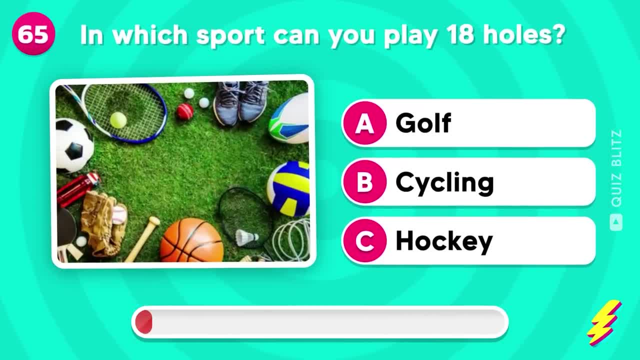 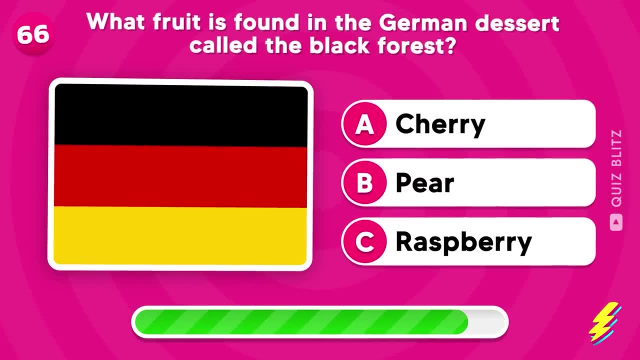 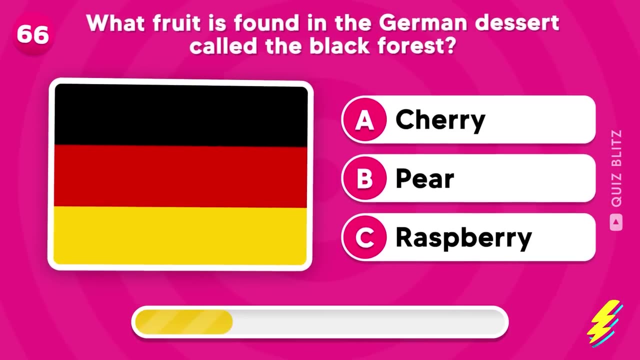 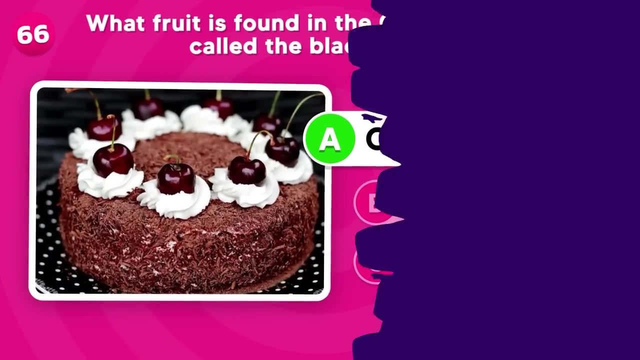 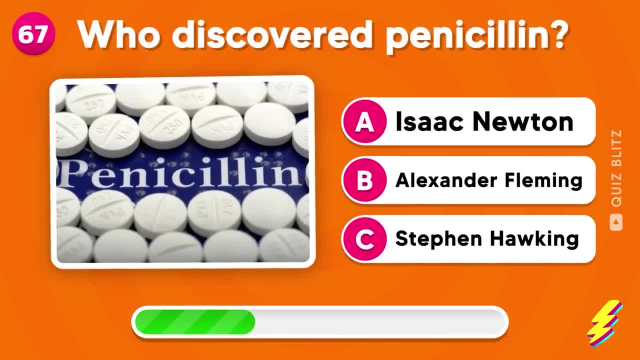 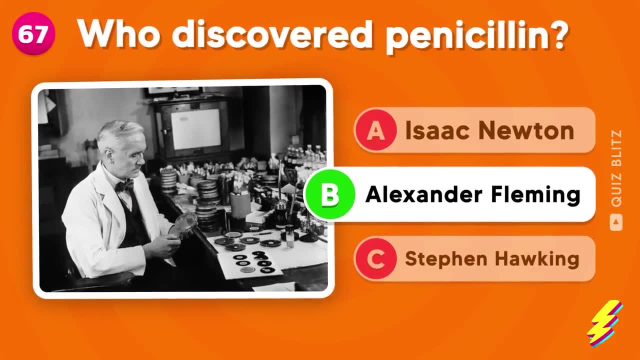 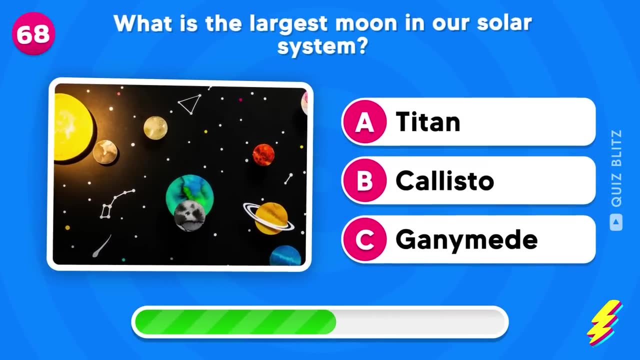 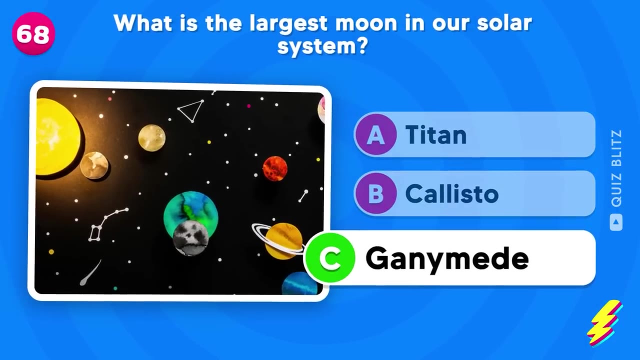 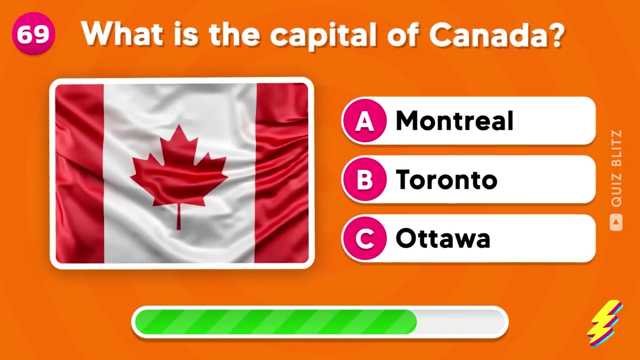 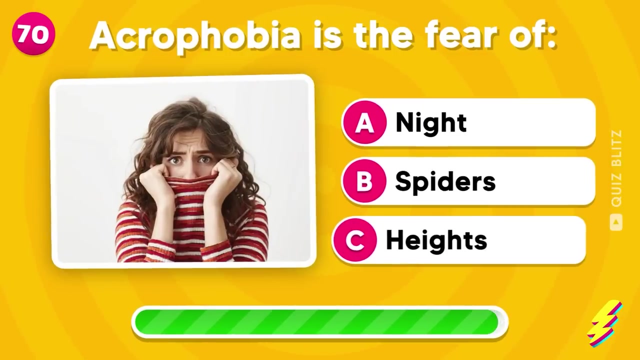 alexander fleming. incredible. what is the largest moon in our solar system? titan, callisto or ganymede? it's ganymede, a satellite of jupiter. what is the capital of canada? montreal, toronto or ottawa? ottawa acrophobia is the fear of night spiders or heights. 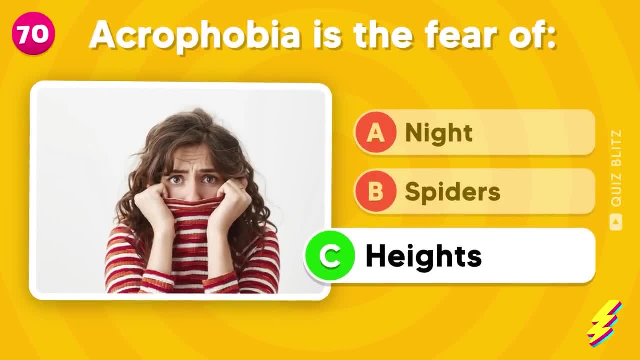 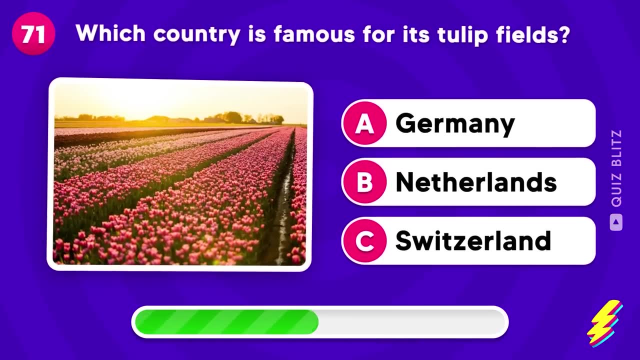 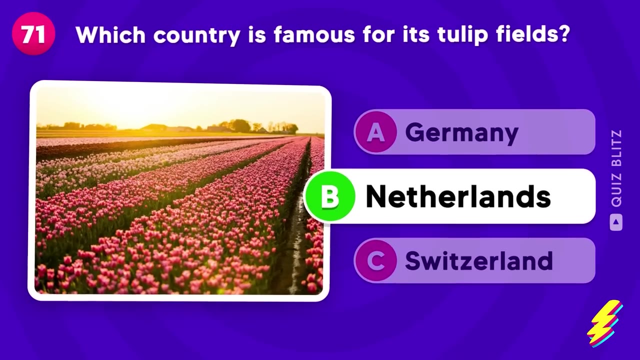 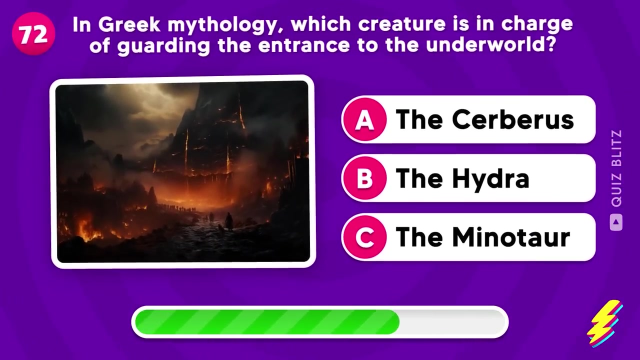 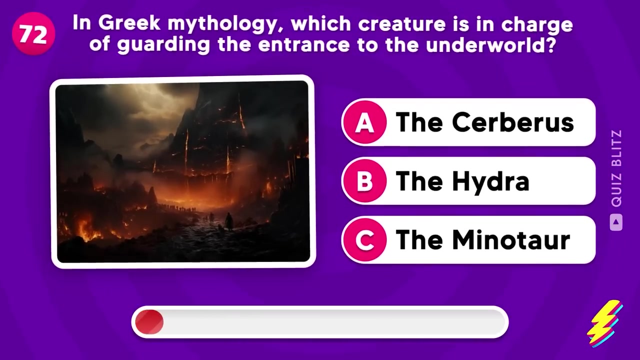 the fear of heights. which country is famous for its tulip fields? germany, netherlands or switzerland? the netherlands. in greek mythology, which creature is in charge of guarding the entrance to the underworld? the cerberus, the hydra or the minotaur? And yes, it's the Cerberus. 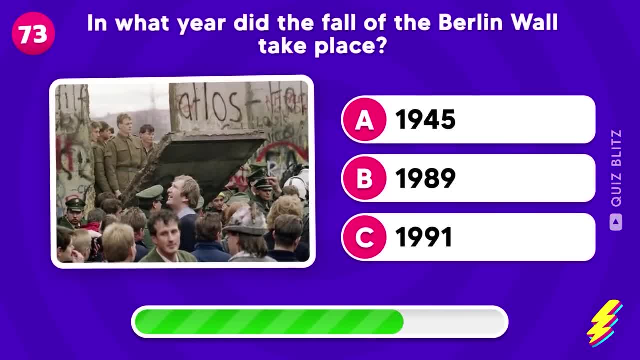 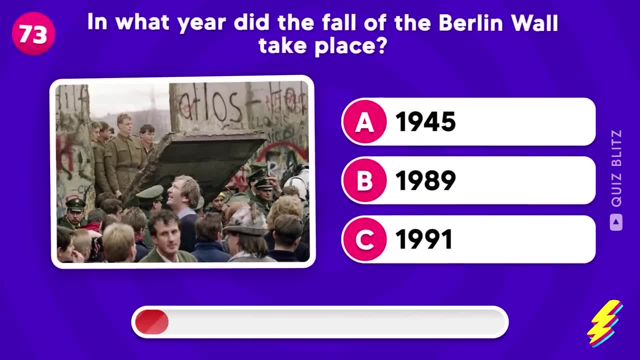 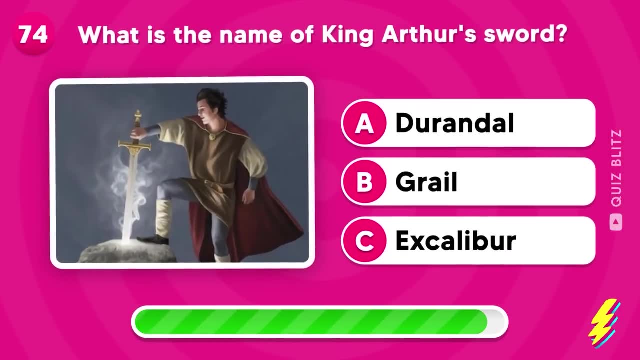 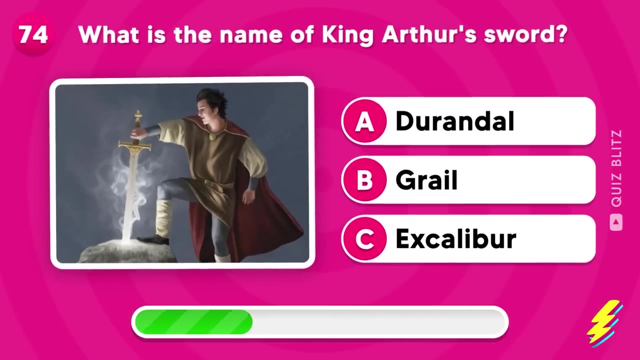 In what year did the fall of the Berlin Wall take place? Answer: A, B or C. It was on November 9th 1989.. What is the name of King Arthur's sword? Durandal, Grail or Excalibur. 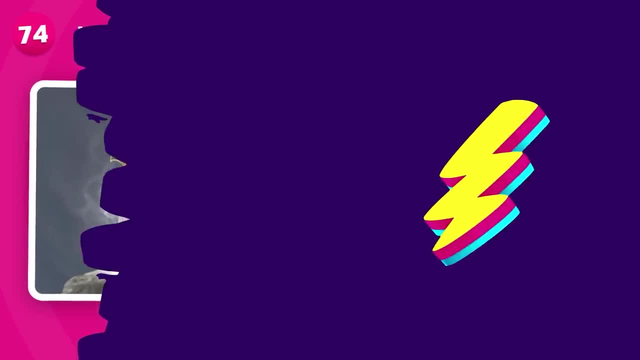 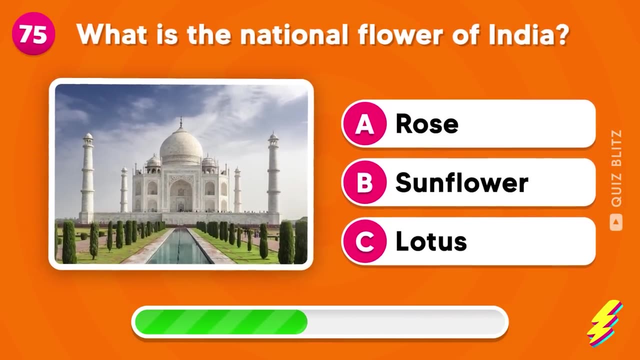 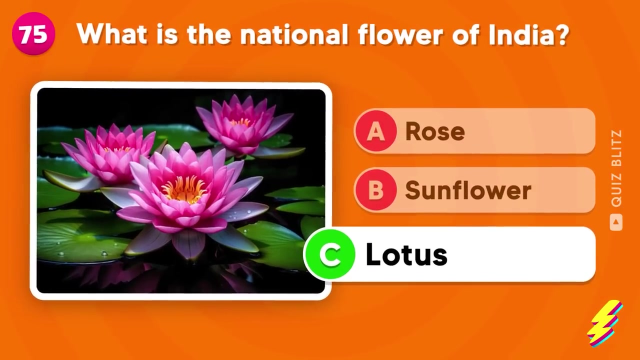 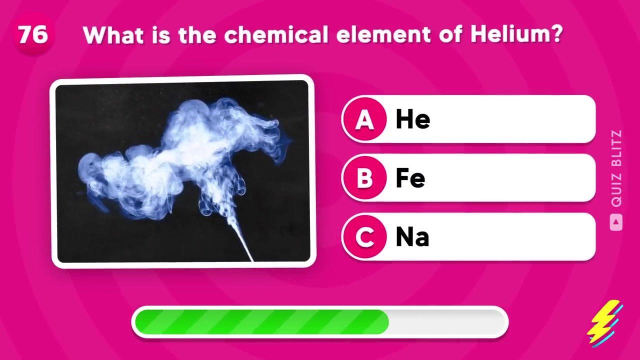 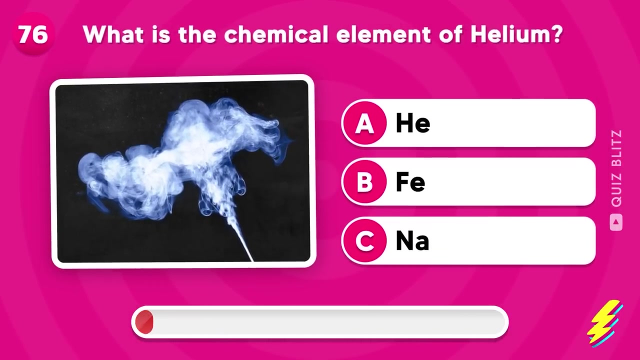 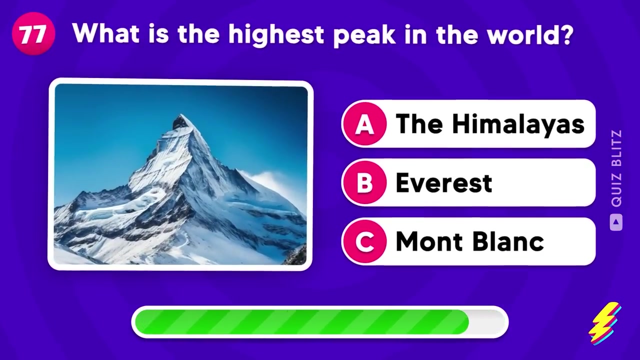 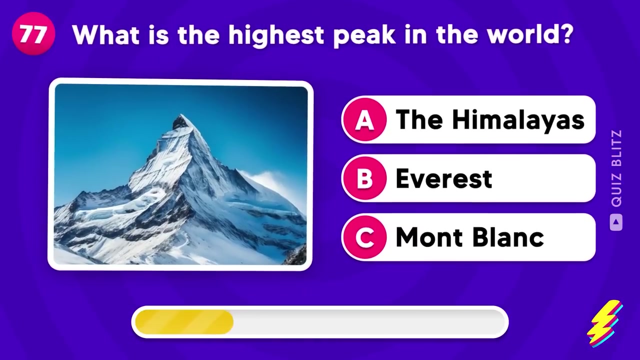 Excalibur. What is the national flower of India? rose, sunflower or lotus, Lotus Lotus? What is the chemical element of helium? H-E, F-E or N-A? It's H-E. Well done. What is the highest peak in the world? the Himalayas, Everest or Mont Blanc? 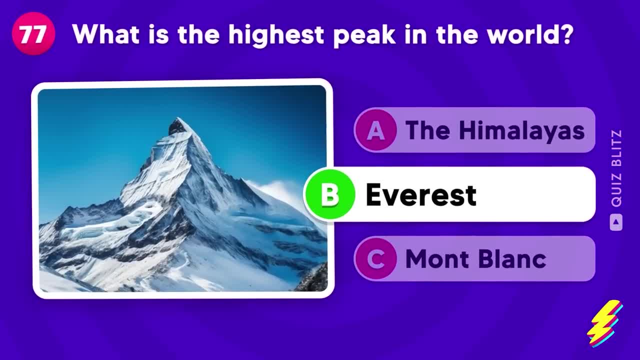 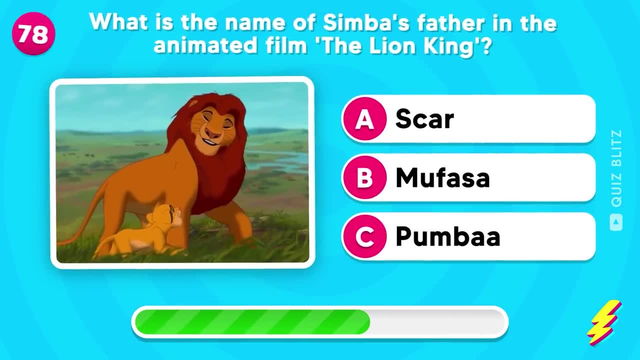 Everest. What is the highest peak in the world? the Himalayas Everest or Mont Blanc Everest? It's Everest with its 8848 meters high. What is the name of Simba's father in the animated film The Lion King? 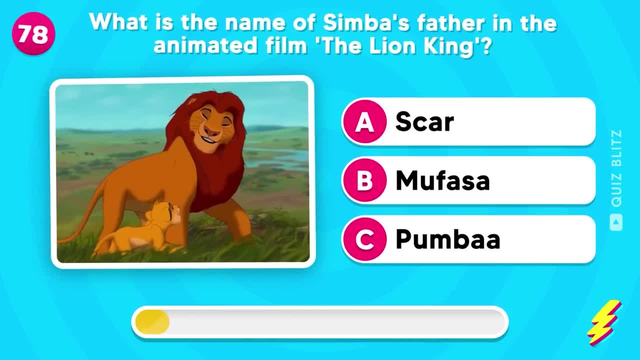 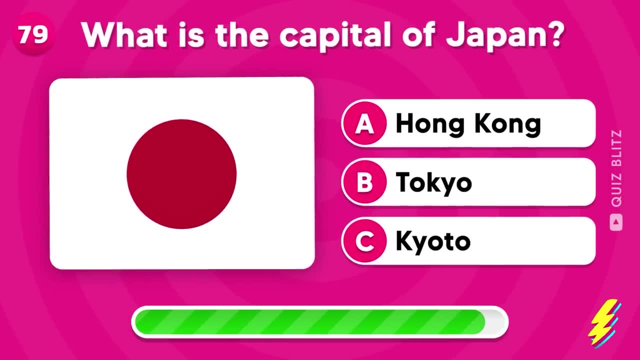 Scar, Mufasa or Pumbaa, Scar, Mufasa or Pumbaa, Mufasa, Mufasa. I loved the Lion King, did you? What is the capitol of Japan? Hong Kong, Tokyo or Kyoto? 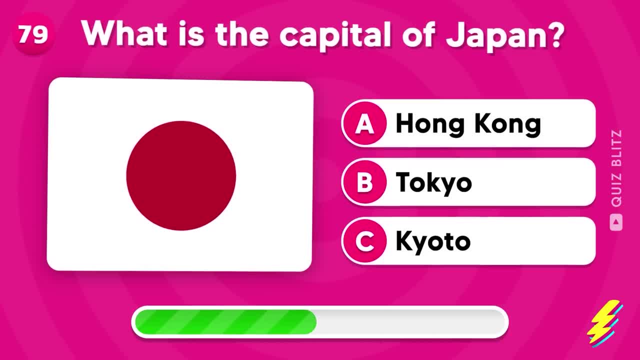 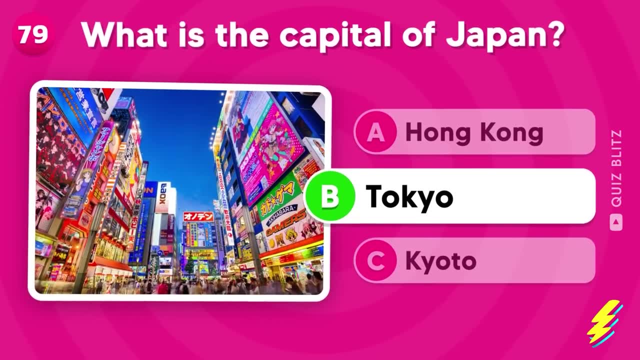 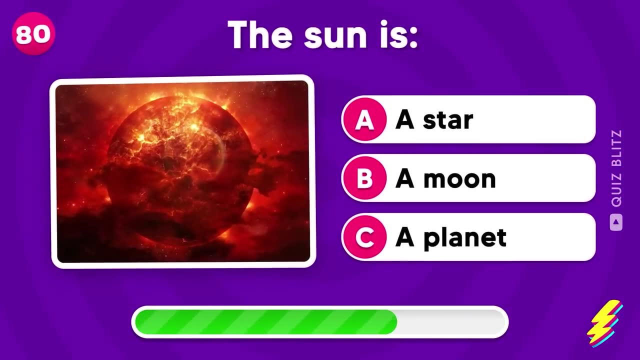 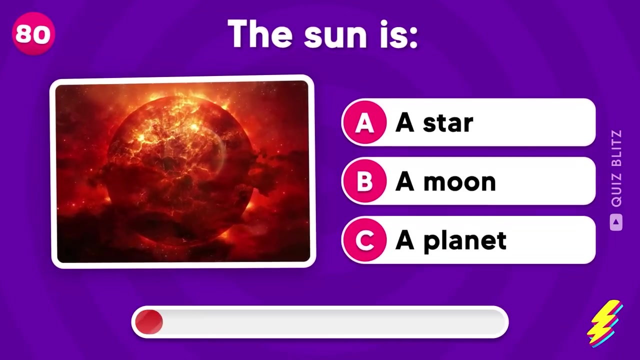 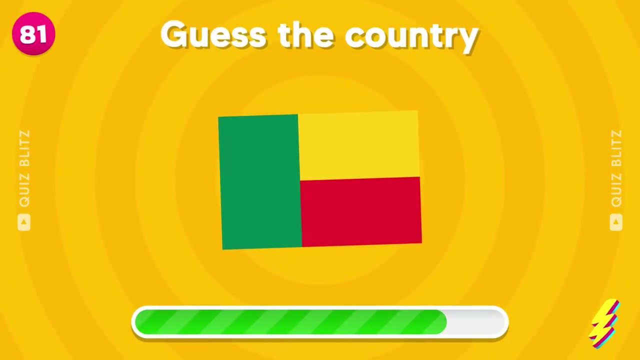 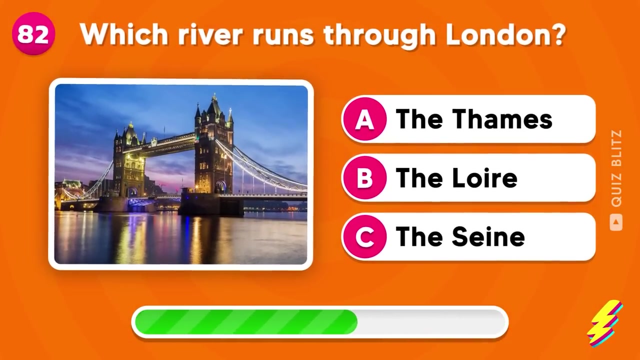 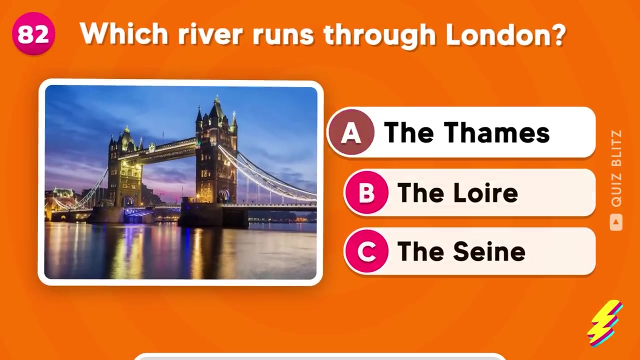 Hong Kong, Tokyo or Kyoto? What is the capital of Japan? Tokyo? the Sun is a star, a moon, or a planet, a star? guess the country? it's Benin, really not easy. which river runs through London? the Thames, the Loire or the same the Thames? 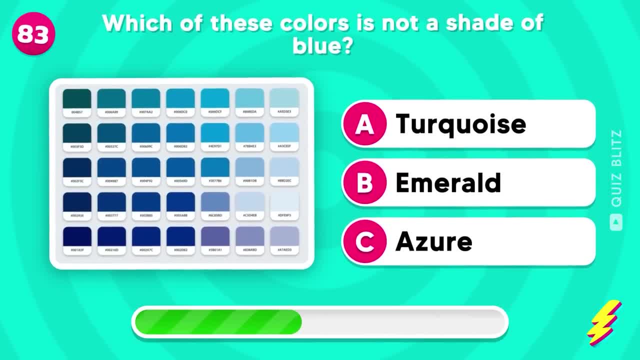 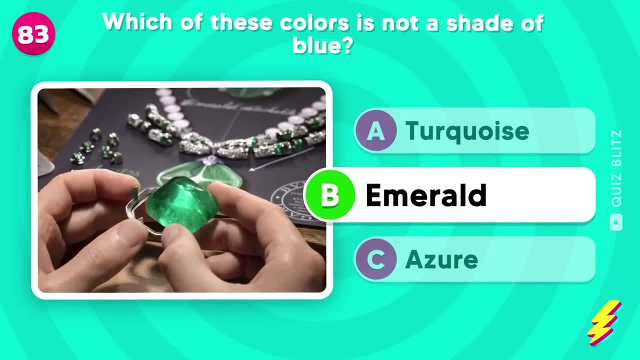 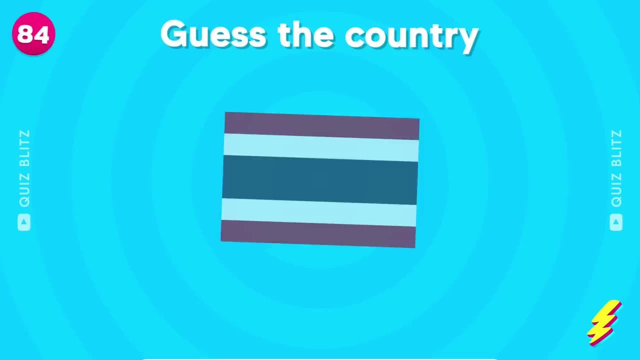 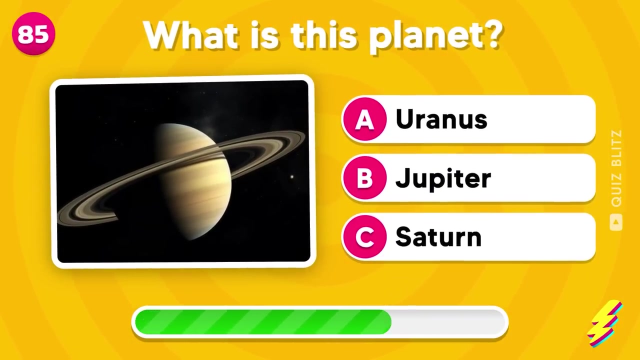 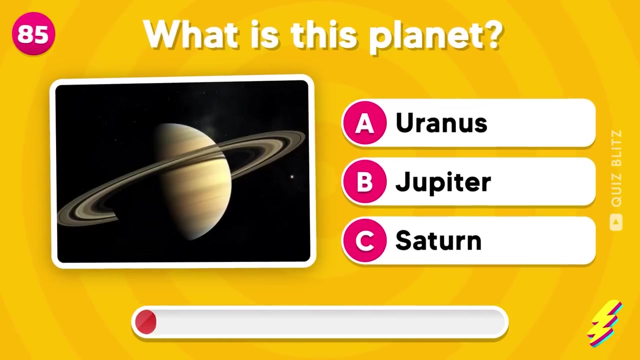 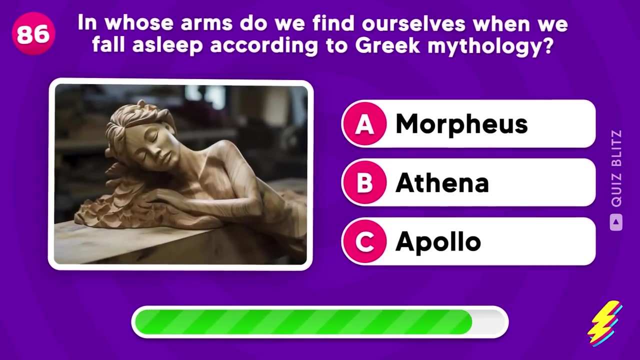 which of these colors is not a shade of blue, turquoise, emerald or azure? emerald refers to a bright and saturated green reminiscent of the color of the precious stone emerald. and this one, yes, it's Thailand. what is this planet? Uranus, Jupiter or Saturn? and yes, it's Saturn. in whose arms do we find ourselves when we fall asleep? 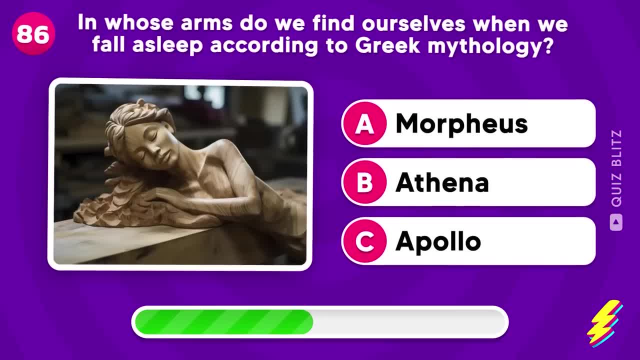 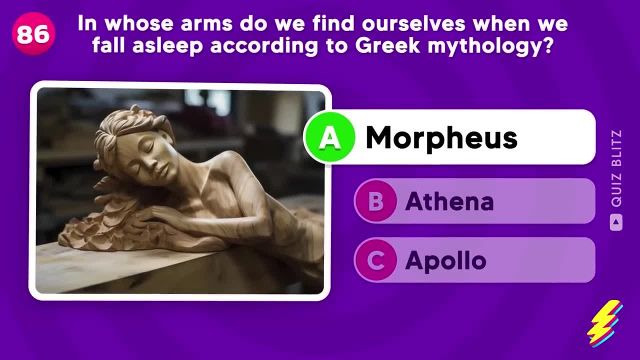 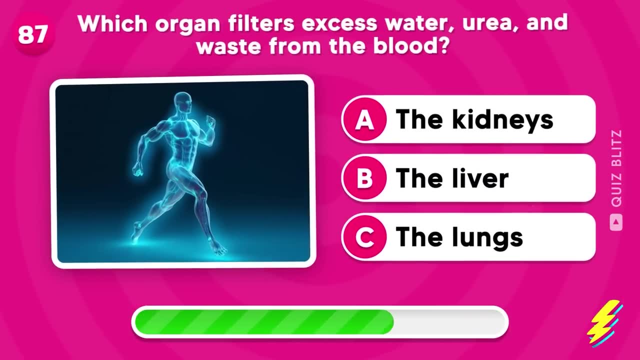 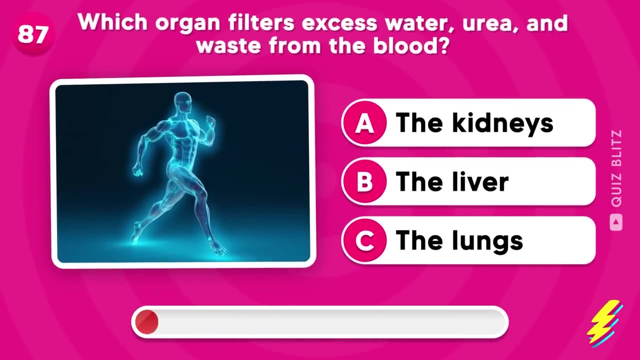 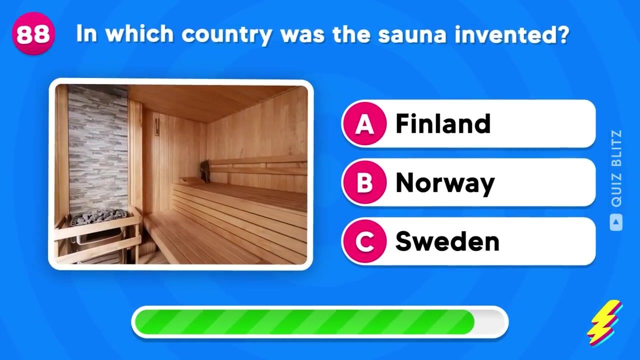 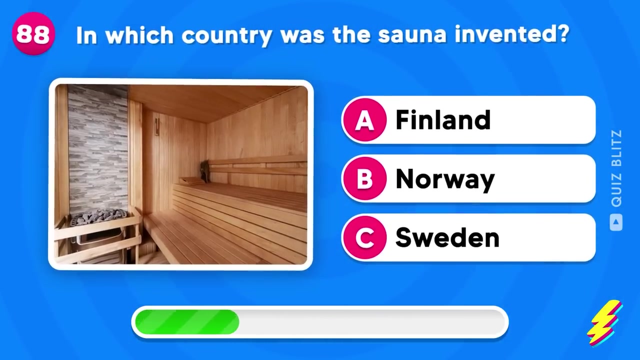 according to Greek mythology, Morpheus, Athena or Apollo Morpheus, that wasn't easy. which organ filters excess water, urea and waste from the blood, the kidneys, the liver or the lungs, the kidneys? in which country was the sauna invented? Finland, Norway or Sweden? it's in Finland. 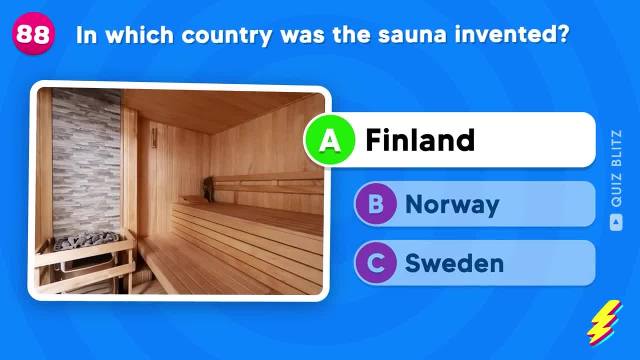 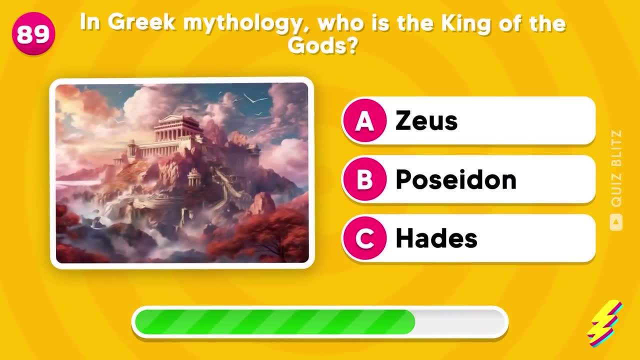 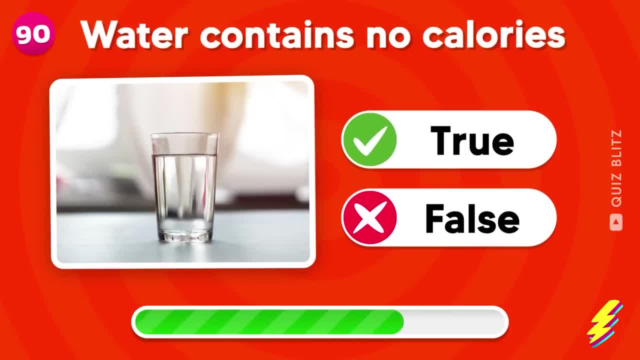 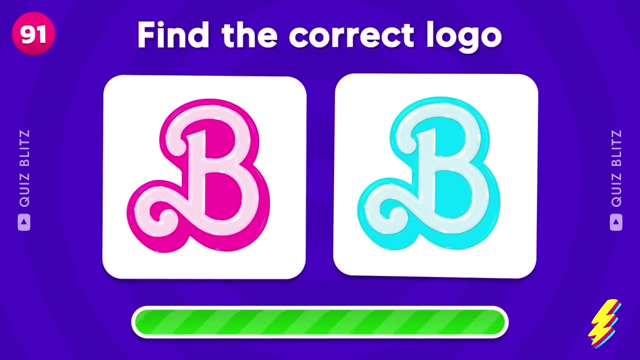 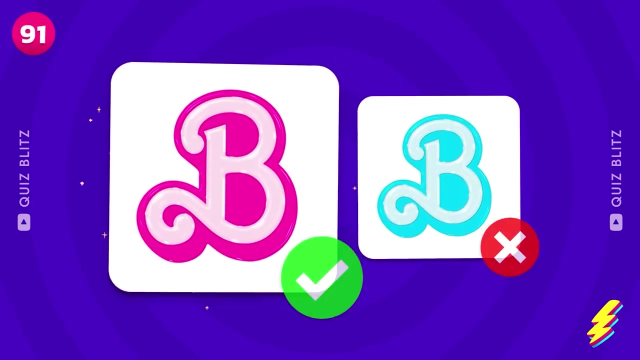 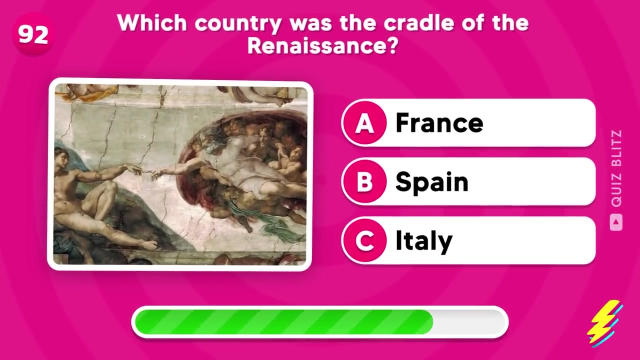 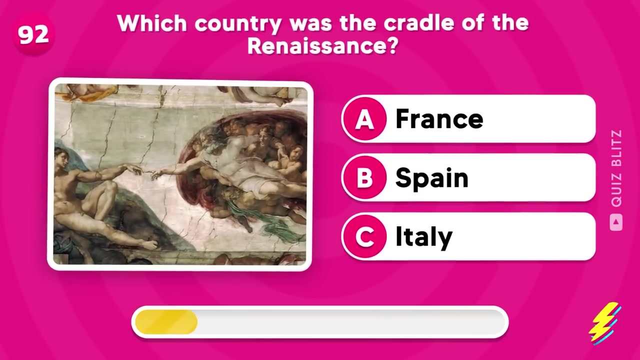 water contains no calories, true or false? i he 2, q s, N, Q 3. What is the real logo of Barbie? The pink one, obviously. Which country was the cradle of the Renaissance? France, Spain or Italy? It's Italy.